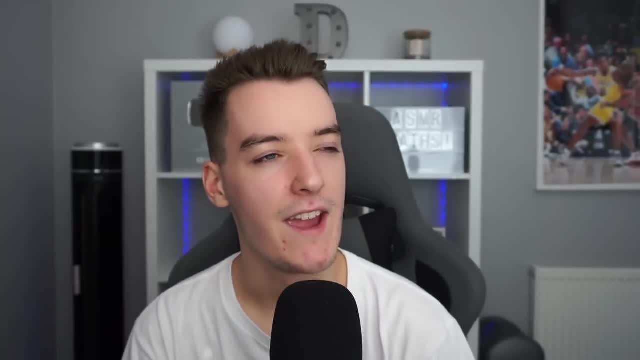 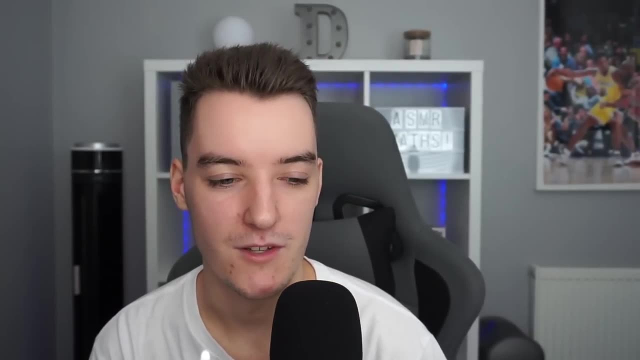 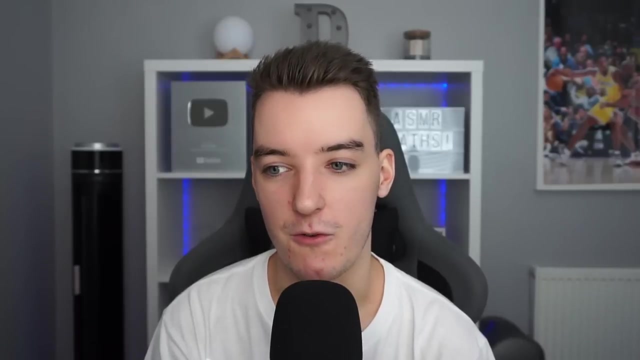 I am really, really looking forward to tonight's video because I absolutely love maths. For those who may be new to the channel, we have done plenty ASMR maths videos in the past. Be sure to check them all out. and the reason being is because, well, I am a recent maths fan. 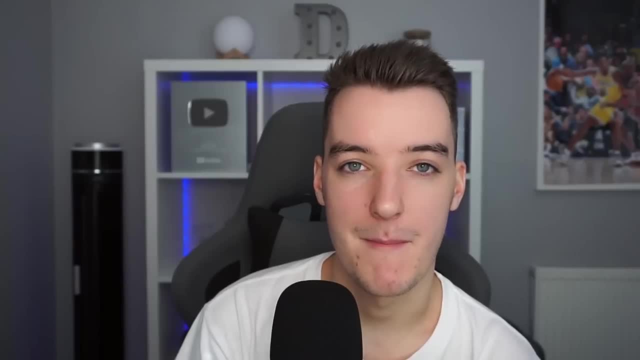 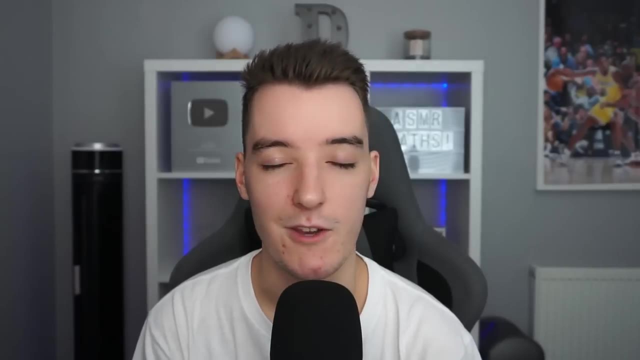 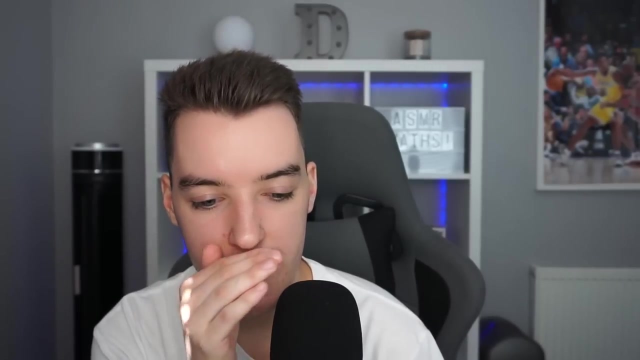 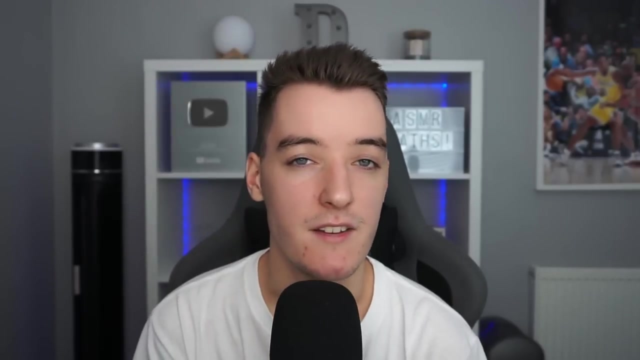 I am a recent maths graduate. I just graduated from a maths degree. I love maths and I really want to go into teaching maths here in Scotland at high school. So in tonight's video I thought I would solve a mixture of maths problems until you fall asleep. 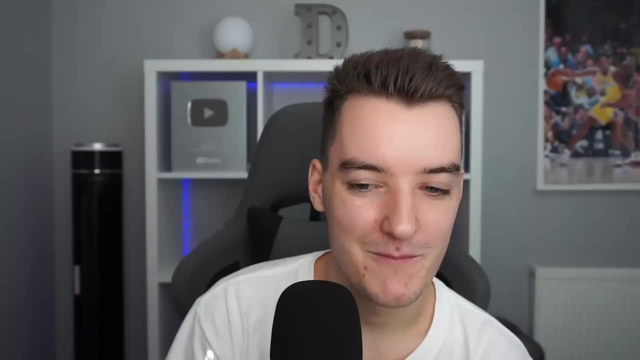 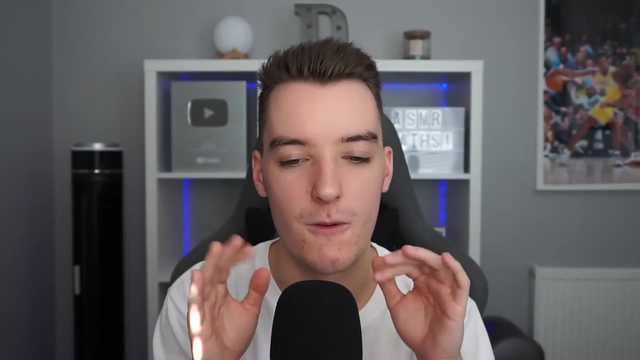 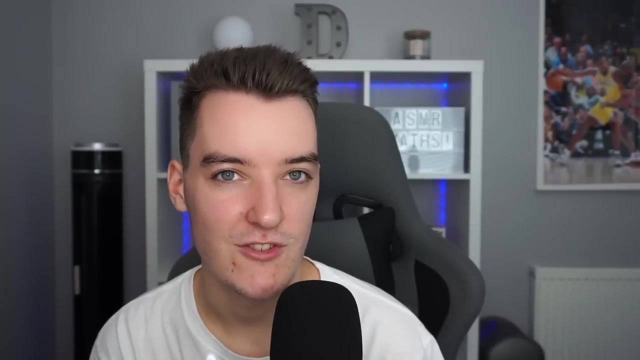 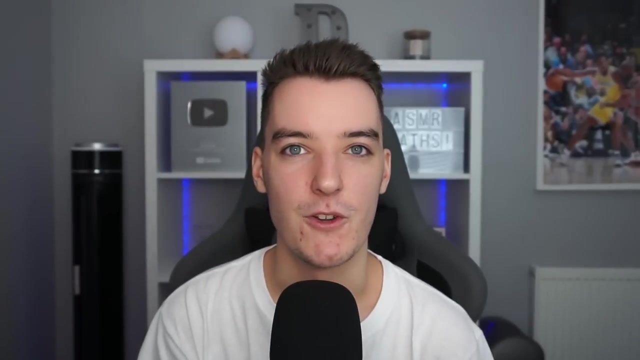 So your goal is to try not to fall asleep whilst enjoying the relaxing ASMR maths, the problem-solving tinkliness, the satisfaction of solving the problems and maybe you like educational maths in this extra-long ASMR video. And so if you do enjoy tonight's video, why not consider dropping it a? 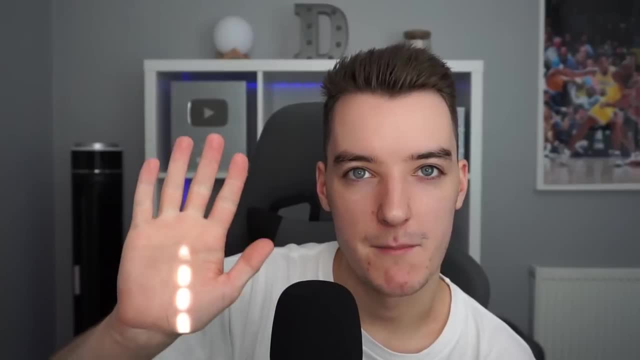 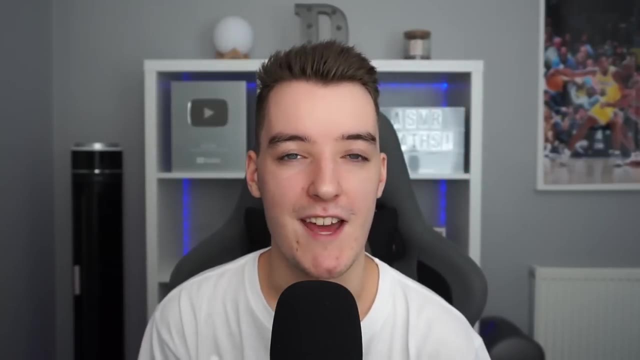 Big thumbs up. Apologies about the light. like reflecting, It's um. I'm recording this during the day, Um, and if you're new to the channel and you're not already subscribed, then why not consider subscribing? It would really mean the world to me. 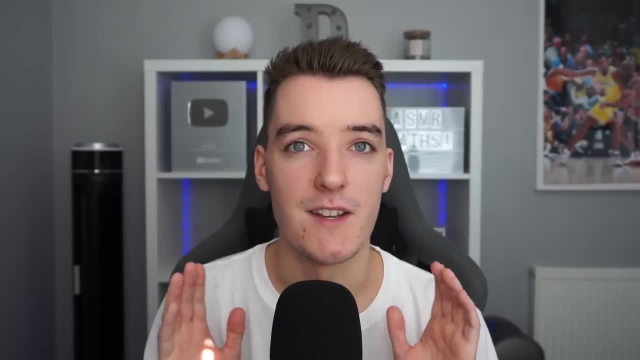 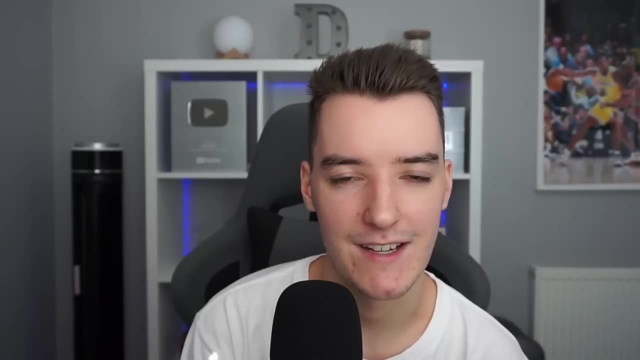 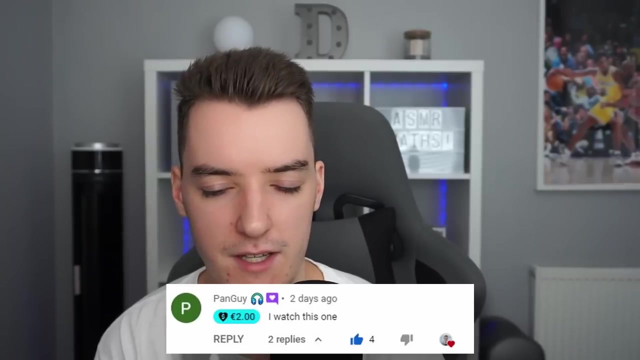 And, uh, real quick, before we get in, I do want to say a massive, massive thanks to one person in particular, and that is PanGuy. PanGuy is one of you, One of our subscribers and a channel member who has just been showing so much support in the comments lately that it couldn't go unnoticed. 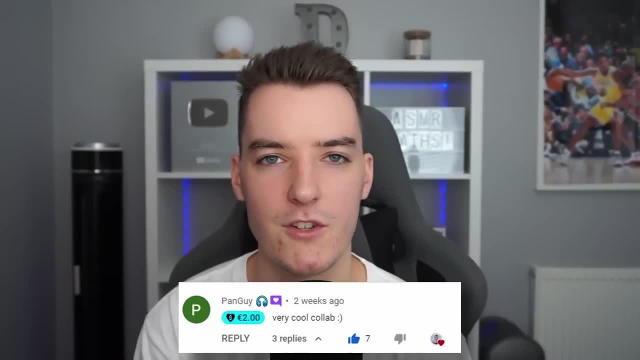 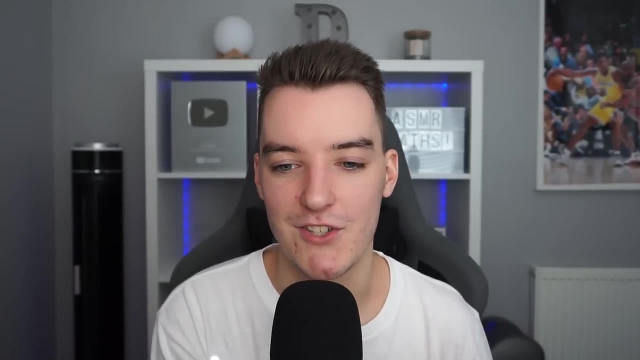 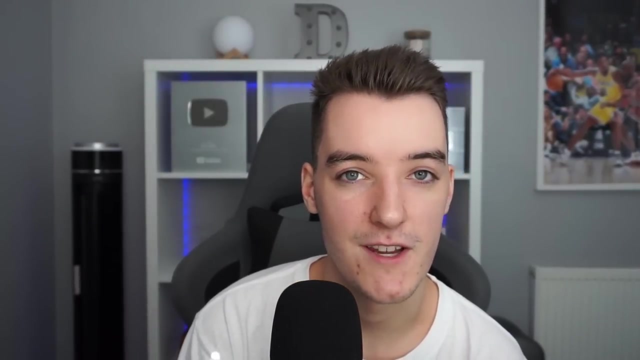 So I want to say a huge thanks to PanGuy and all their super thanks lately. This is just my way of saying a super thanks back to them, so I really appreciate it And uh yeah, without further ado, please sit back, relax and enjoy this ASMR maths video. 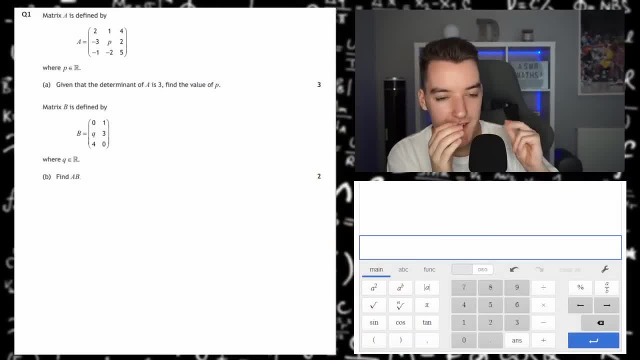 Alrighty, everybody. So this is my little setup. I've got going for this video, Um. I hope you guys like it. It's kind of similar to um, the last maths video I did here on the channel. You can see we have the questions over that way on the left. 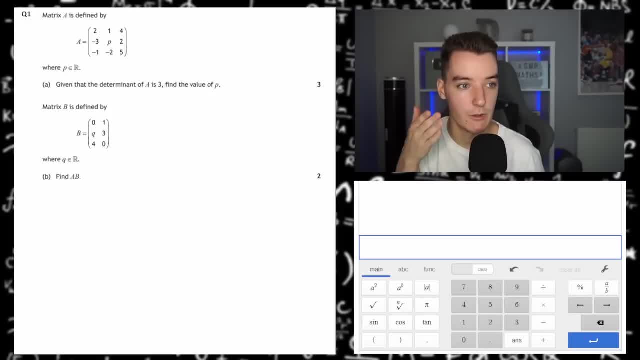 Uh, so if you see me kind of looking down here, that's me actually looking at the questions as I do them. Um, then you have my face up here, a little face cam, and then right down below me we have a calculator, um, a scientific one. 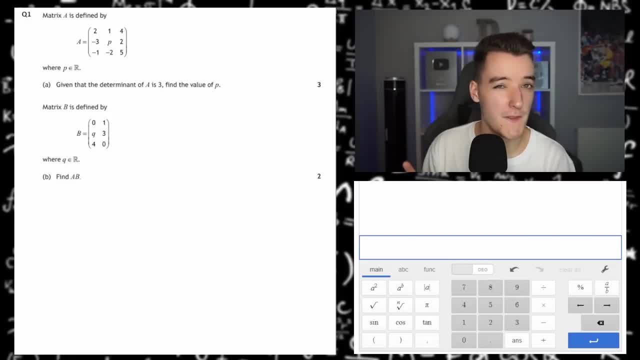 Um, although I will let you know that not all of these questions I'll be allowed to use a calculator. In fact, the questions we have tonight are compiled from a combination of complexities, so some questions might be slightly harder than some Others, from a different level, um, as they were picked out from or by my girlfriend, so big thanks to her for making this for us to do. 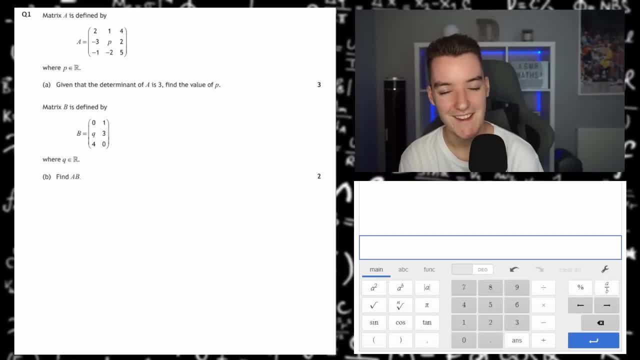 She said it should be possible for me. so here's hoping we do alright, and here's hoping that you guys do enjoy them, whether you understand the questions or not. and, um, yeah, I think, without further ado, we will just get started. 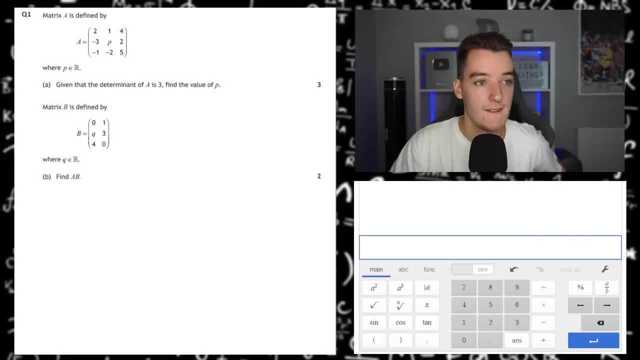 Subtitles by the Amaraorg community. This first question, which I've been told is a non-calculator, looks to be a little bit of a matrix question. so we're going to be doing some algebra, um, and I love matrices, so this is going to be a fun question here. 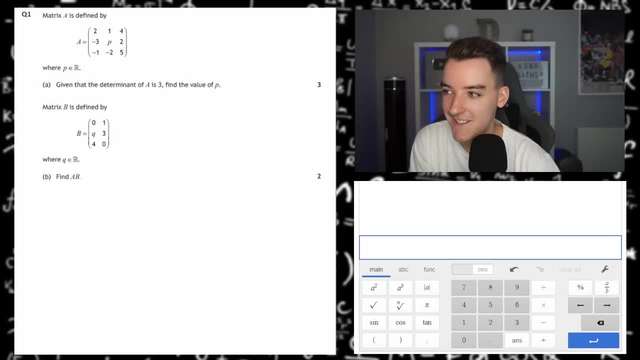 Now it also tells us the marks, because all these questions were actually from a- uh wait, is this working? Yeah, All these questions, All these questions were actually from a um pass paper from exams that we have here in Scotland. so you can kind of gauge, um, what you need to do in order to get all the marks, but that shouldn't make too much of a difference. 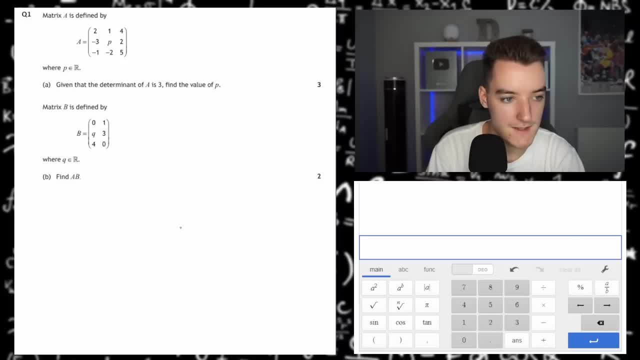 Anyway, let's just get started with part A to this question, uh, which says matrix A is defined by: And then we have this 3x3 matrix with B, which is entry 2 to the middle entry um is some real number that we don't know um, but part A says: given that the determinant, the determinant, the determinant determinant of A is 3, find the value of B. 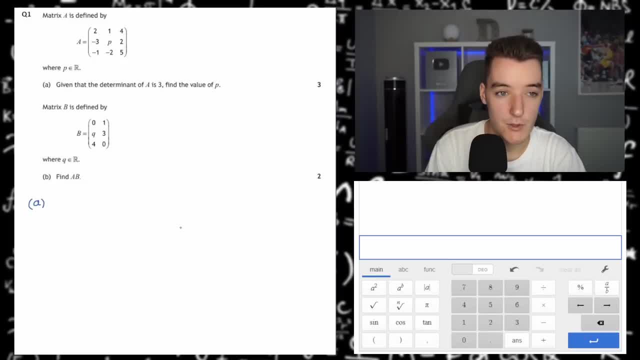 Okay, so I am going to do this By actually working out the determinant of A, because I feel if I do this it will involve B in some way, some sort of algebraic expression, and if we equate this to 3, I'm assuming we can uh rearrange and solve for B in that sort of sense. 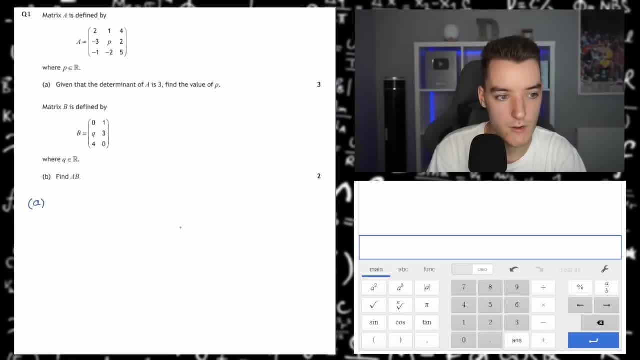 So for those who don't know, determinant of a 3x3 matrix, you use this process where you take the top left most entry, which is 2.. But let's actually write that the debt of A, which is technically 3, is equal to 2, multiplied by the determinant of the bottom 4 entries. so you kind of score out if you imagine the row and the column that the 2 is in. 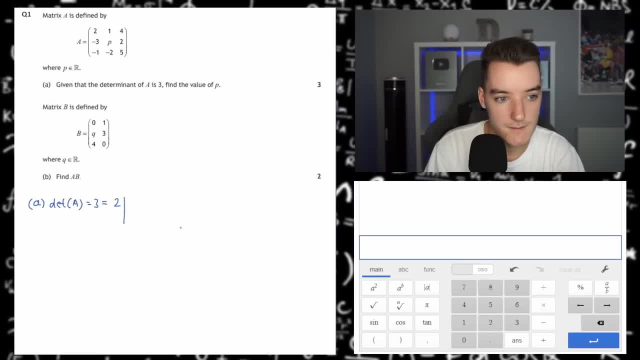 So that matrix now becomes B 2, minus 2. And 5.. And then you do the same, but you move over to the 1, and you stick a negative in front, because you alternate symbols when you do this process. 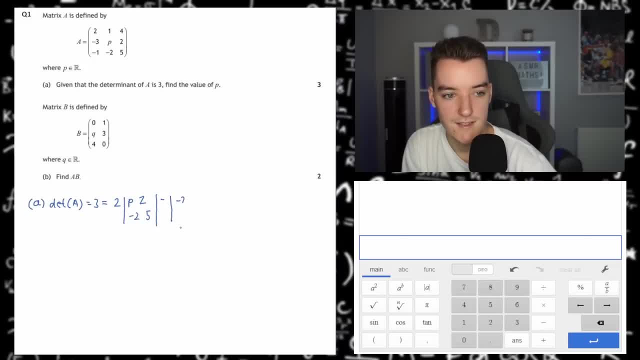 It's a bit weird and it doesn't make too much sense, even to me. So now we've got 3, uh, minus 3,, 2, minus 1, and 5.. And then you do plus. Now the reason I didn't write the 1 is because, well, that's just the same as 1 times. 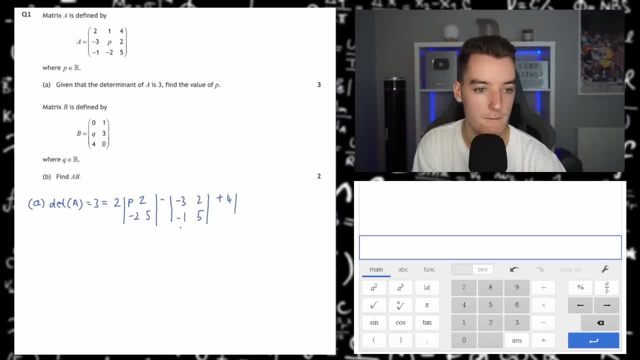 the negative, you know. So now we have plus 4, times it's going to be minus 3, B minus 1, minus 2.. And all we do now is just solve this determinant. so we're going to have 3 is equal to 2, and then to work out the determinant, to determine the determinant of this matrix, we do B times 5, which is 5B. 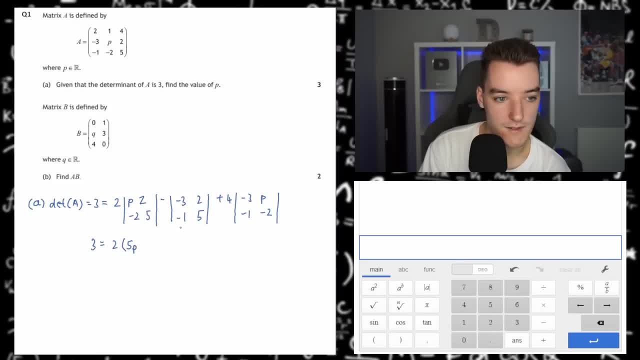 And we subtract the opposite ones. so subtract minus 4,, which is plus 4.. Moving on to the next one, we have minus 15, minus minus 2,, which is plus 2.. Moving on to the last one here: plus 4, minus 6, minus minus B, which is plus B. 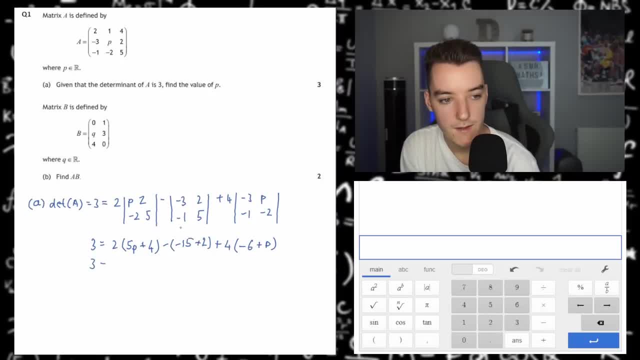 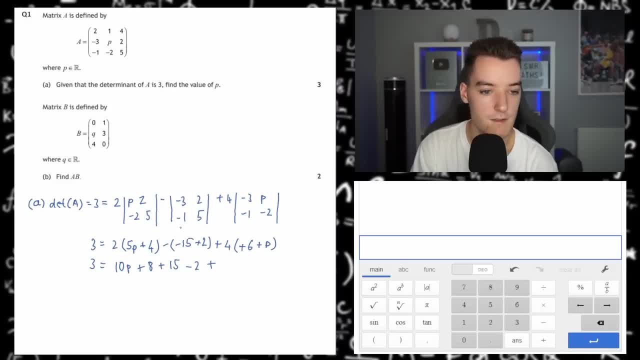 Uh plus uh, 24, plus B. Yes, that looks right. Um, so, uh, no plus 4B. Sorry, my brain is still trying to wake it up. Um, I've recently woken up. 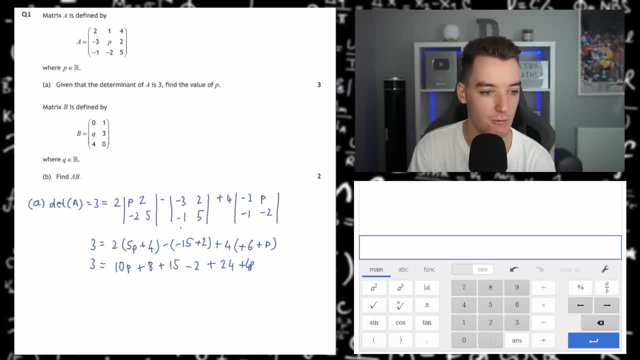 Uh, plus 4B. Okay, now we're all good. So rearranging: now we get 3 is equal to we've got 14B, and then 8 plus 15 is 23,. minus 2 is 21,. plus 24 is plus. 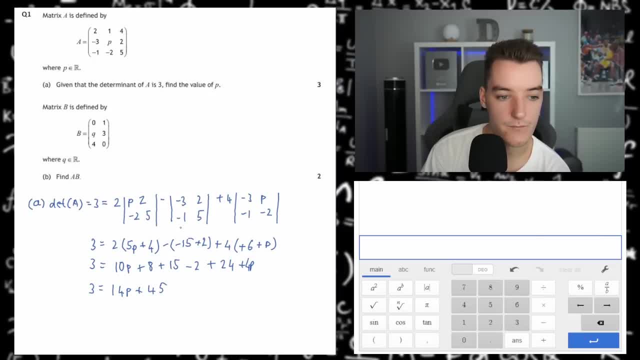 45, and then rearranging gets 14B is equal to minus 42,, which is nicely divisible by 14,, which gives us B is equal to minus 3.. And so we have determined the value of B, which is exactly a real number. so that is perfect. 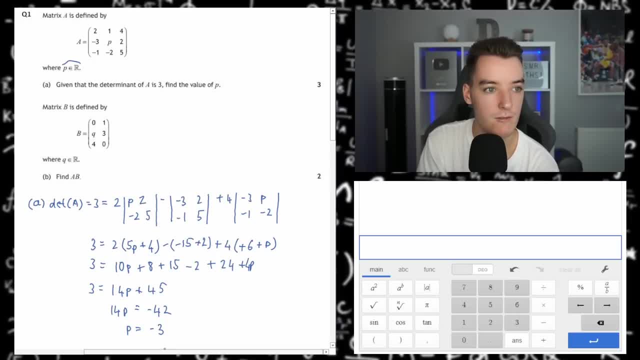 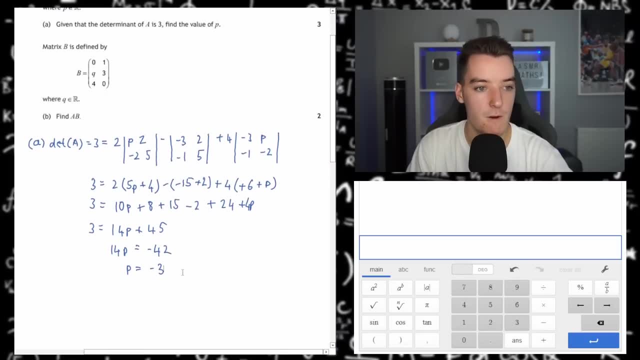 Uh, as it told us, you know, B is a a real number, so that's all looking pretty good. Let's move on to the second part of question number one, which is matrix. B is defined by: we've got this: 2 by 3, um, 3 by 2 matrix. 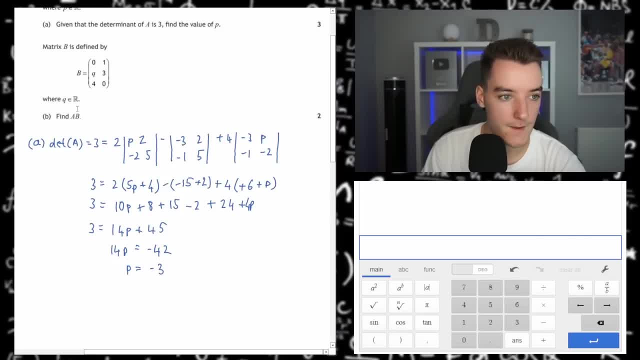 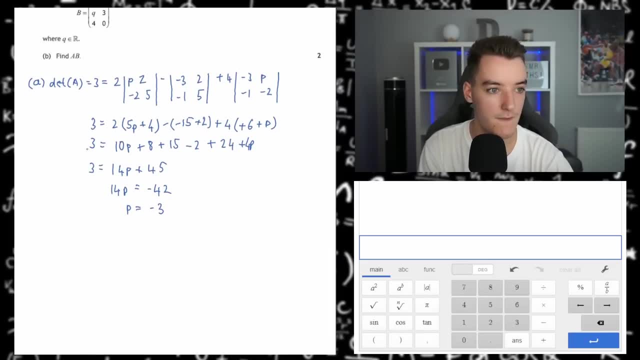 where Q is some real number, Find A times B. so we're multiplying matrices this time. Okay, so in this case B is going to equal. oh, no, sorry, AB is going to equal. well, we've got the 3 by 3 matrix in part A. 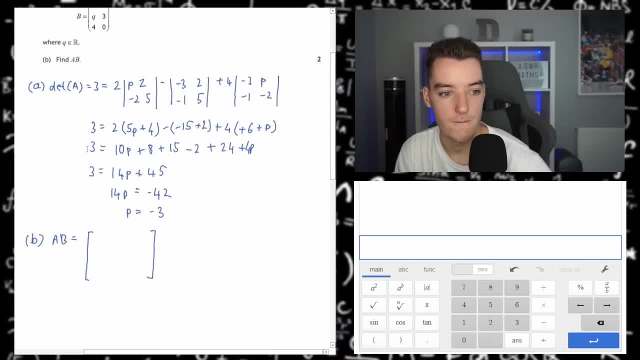 which I'm going to forget. so it goes 2, 1, 4 along the top: 2, 1, 4, well, we know it's minus 3, minus 3, because we know now that B is minus 3,. 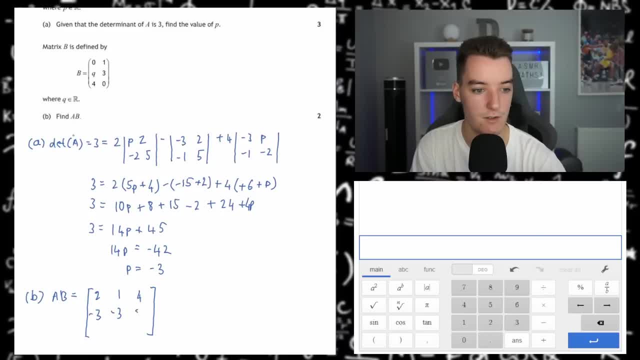 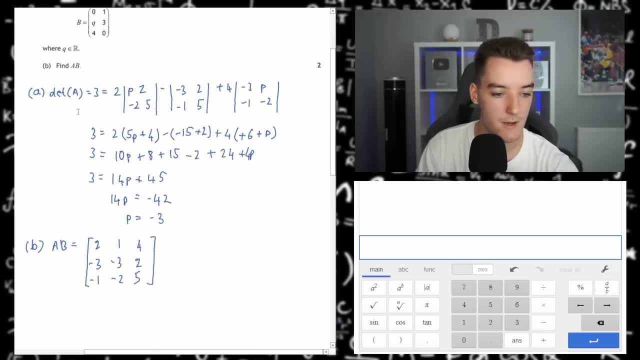 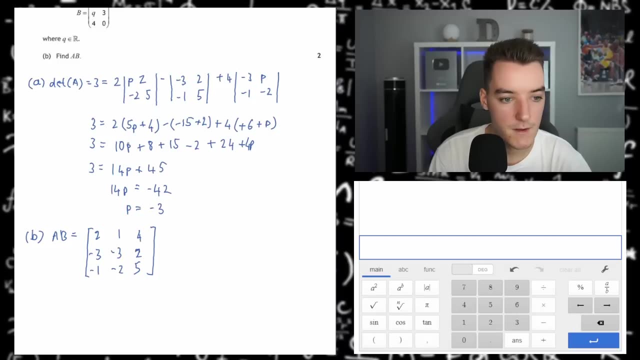 so, then, the last entries are 2, minus 1, minus 2, and was it 5,? I believe Yup. so that's A, And we are multiplying it by B, which is a 3 by 2. that goes 0, 1, Q, 3, 4, 0,. 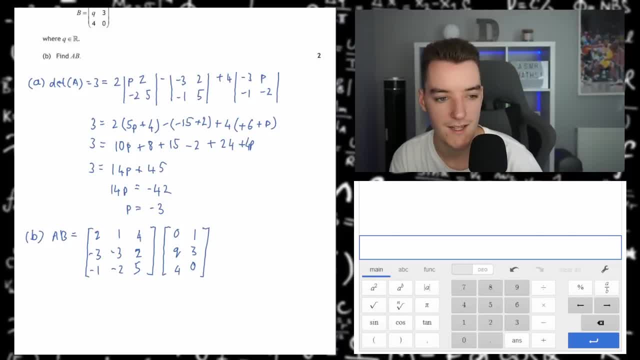 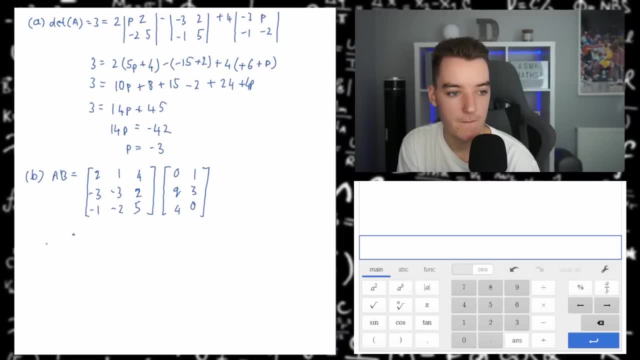 and it's quite nice. There's a few 0s in there. that's probably going to make it a little bit easier to solve, So let's multiply these together as the birds chirp away in the background. I apologize. 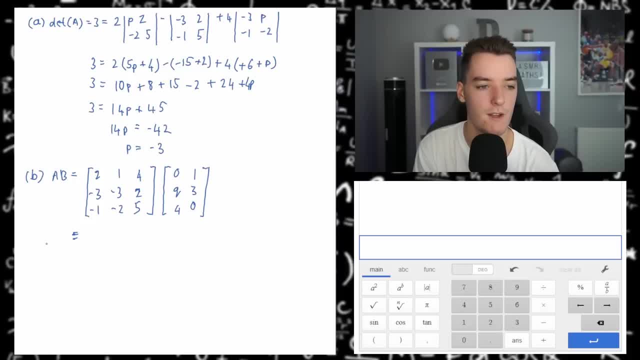 Maybe you like it- I don't know. It is daytime that I'm recording this. So we're going to have a 3 by 2 resultant matrix, because B is a 3 by 2, so it's going to look. 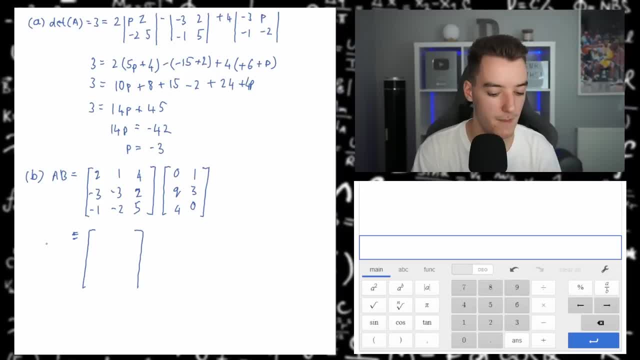 something like this. it's going to be a little. actually, I'm going to leave myself more space because we're going to have some plus or minus Qs involved. So we're going to take the top row and multiply it by the first column, each corresponding element. 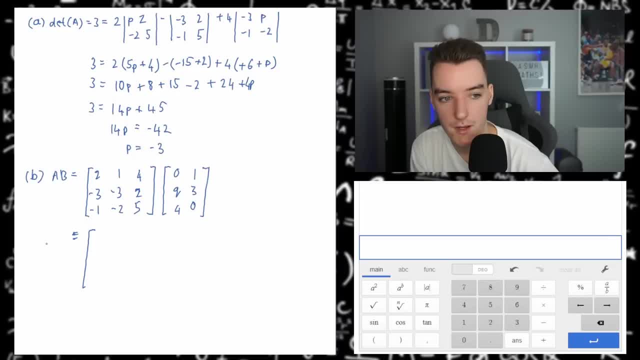 so 2 times 0 is 0, then we're going to plus 1 times Q, which is Q, and then plus 4 times 4, which is plus 16.. Then the next entry below it, we take the next row, minus 3,, minus 3, 2, and multiply it by this column: 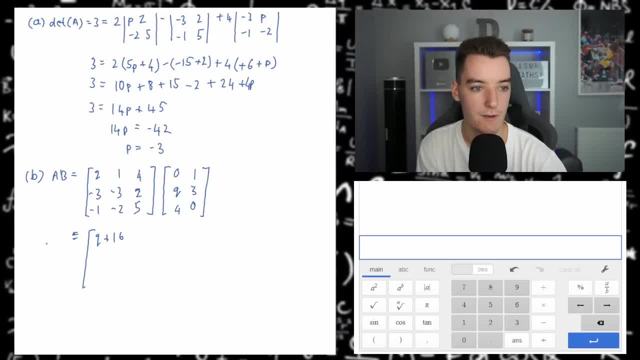 which is 0, minus 3Q plus 8,, I believe, and then the last one is going to go 0, minus 2Q plus 20.. And then, because there's no Qs in this next column, they're all going to be numerical entries in this second column for this matrix. 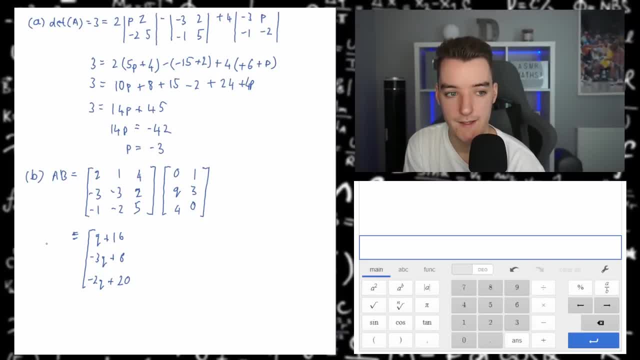 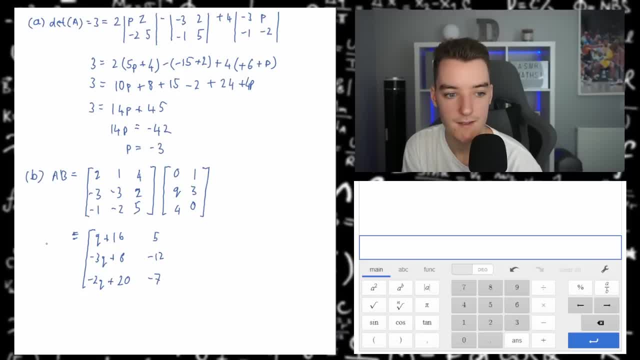 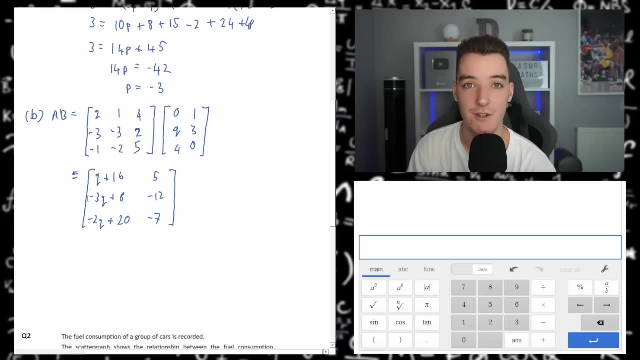 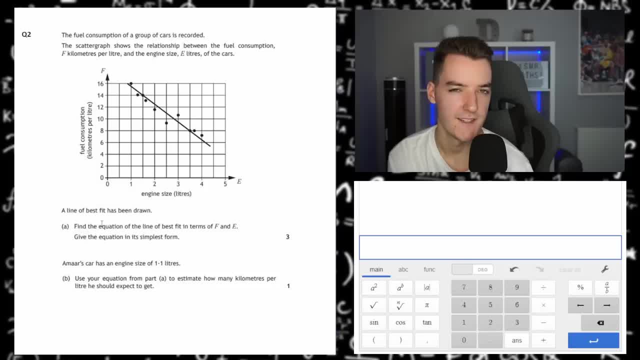 Okay. so question number two. this one is also non-calculator. It looks to be a bit of geometry by the looks of things. We have some sort of- Or maybe- statistics. i'm not too sure yet. let's take a look at it. the fuel consumption of a group of 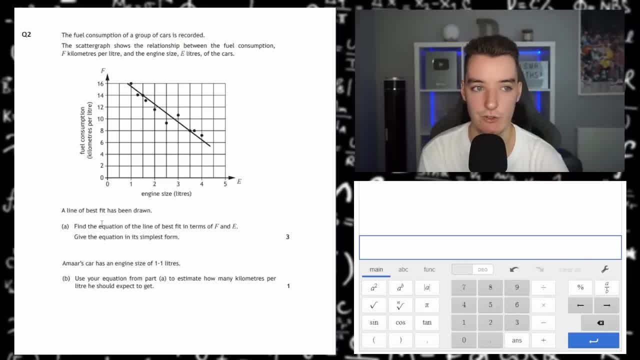 cars is recorded. the scatter graph shows the relationship between the fuel consumption, which we have on the y-axis in f, kilometers per liter, and the engine size, which is the x-axis in e liters of the cars. as you can see all the points which have been scattered across. 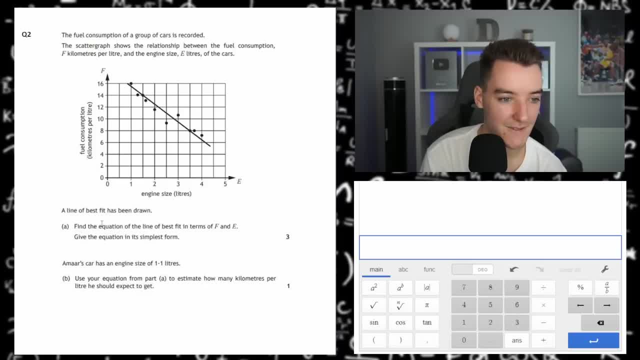 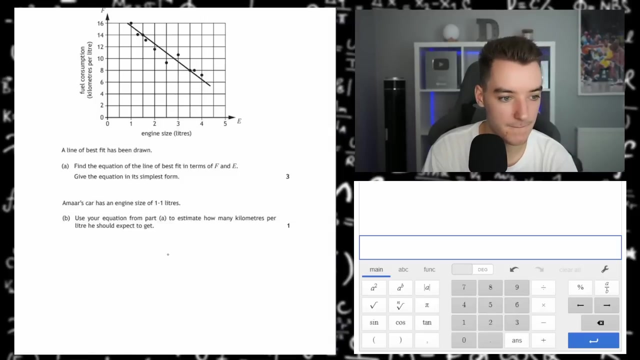 and very nicely. there has been a line of best fit drawn, so that's pretty useful. part a says: find the equation of the line of best fit in terms of f and e. we can do that, okay. so let's start part a, which is worth three marks. so to find the line of best fit. 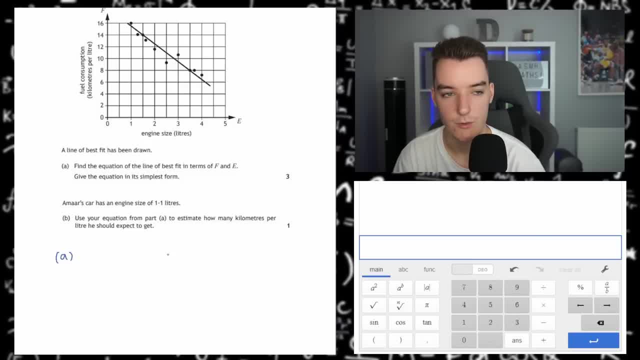 well, if you're ever finding the equation of a line, you need um some points on the line, the gradient, uh. and a point on the line we have, both technically, because we can work out the gradient which we can see by going down here. i'll try and draw it in going down here. 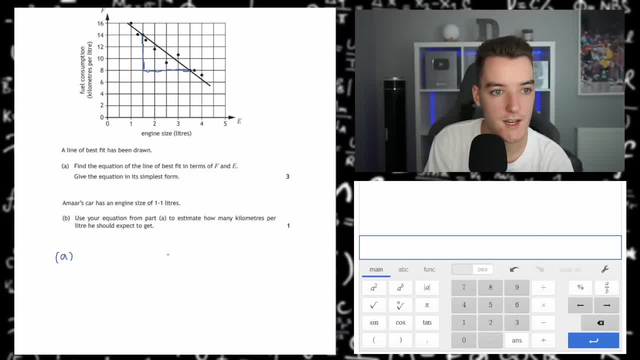 and going down once more, going across, oh my shaky hand, going across. here we can see our gradient. Well, this point here is the point 14 on the y-axis, And to get down here, it goes down to 8. So 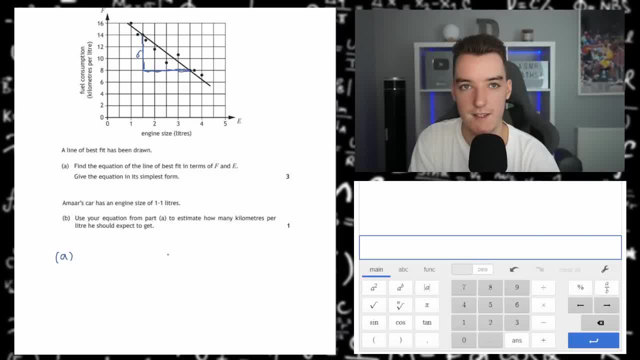 it goes down 6.. Each box is worth 2.. It actually goes down minus 6. technically. That's very important. And then it goes across from 1.5 to 3.5.. Okay, not so bad, It goes across 2.. 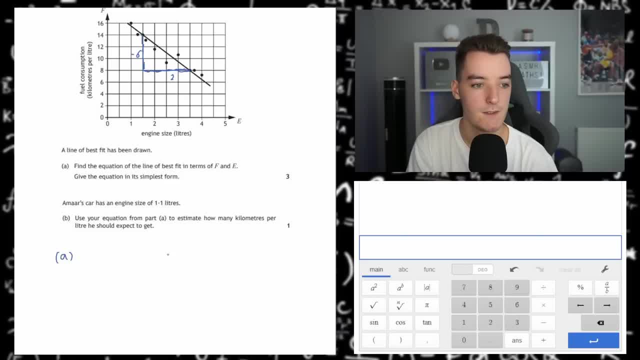 So each box is 0.5.. So the gradient M is equal to minus 6 over 2,, which is equal to minus 3.. I don't know, I don't know why I thought about that for so long. Okay, so we have our gradient Now. 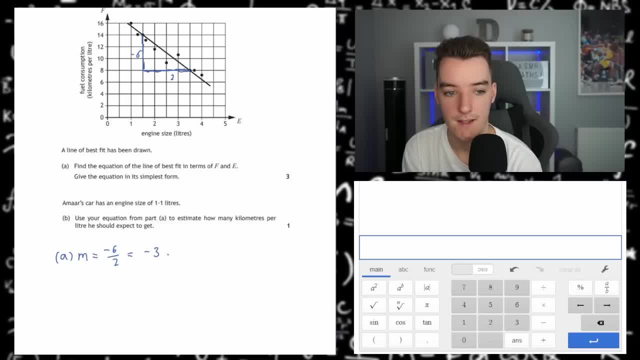 we just need a point on the line, which we do have. Let's take the point, Let's go for 1.514, because now we can input that into the equation: y take b equals m, x take a. this is just a very classic equation. In our case, y is f And a and b are these values? 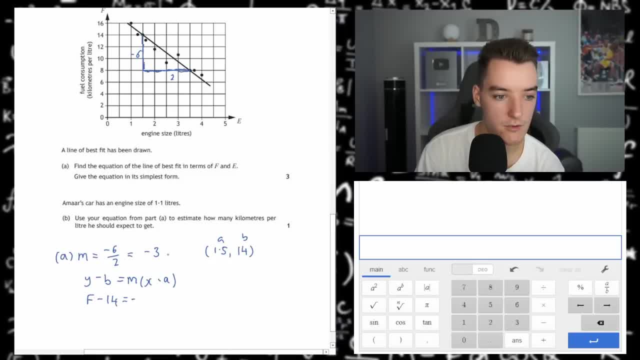 So b is going to be 14,, which equals minus 3.. And x, in our case, is e Subtract a subtract 1.5.. Now, if you bear with me, I need to quickly clear my throat. Apologies about that. So. 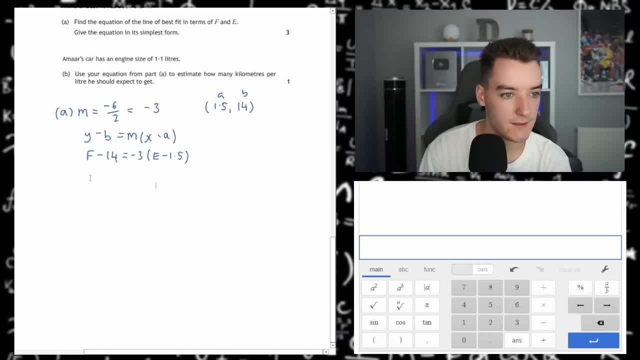 next, we're going to rewrite this just to make it a bit easier. So let us multiply everything by, or let's just multiply everything through, So we get f minus 14 is equal to minus 3e, And then minus 3 times minus 1.5 is going to be plus 4.5. 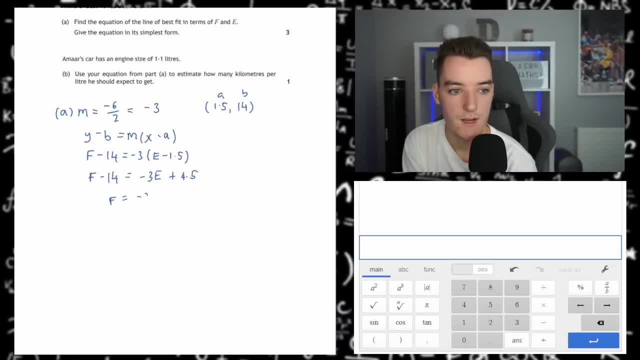 So then we get: f is equal to minus 3e, and then add 14 to both sides, we get plus 18.5. very nice indeed. and that is our uh equation of the line of best fit in its simplest form in terms of f and e. 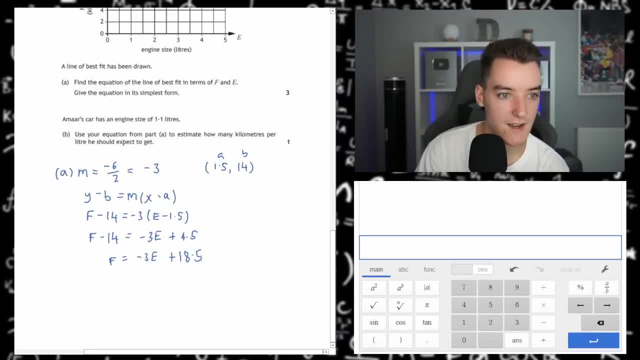 part b says that a mars car has an engine size of 1.1 liters. use your equation from part a to estimate how many kilometers per liter he should expect to get. so if his engine size, if e- is 1.1, we're basically trying to work out. 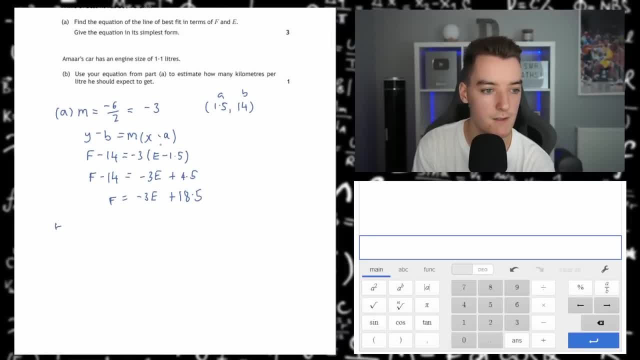 what f is. so that's pretty nice. so b will put: when e is equal to 1.1. sometimes we write this as just e 1.1, but i i won't do that for this. so when e is 1.1, f is going to equal minus 3 times 1.1 plus 18.5, which equals minus 3.3 plus 18.5. 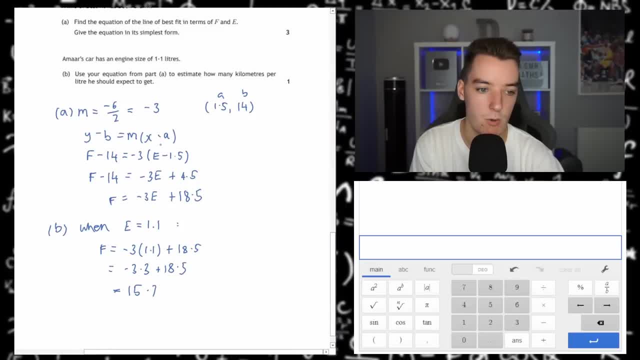 which is 13.2. and oh, we don't forget our, is it kilometers per liter? i believe kilometers per liter. nice, so that is going to be our final answer for part b in question two. so pretty fun question there. i like the concept of the sort of cars and uh yeah, not too bad. let's go into question three. 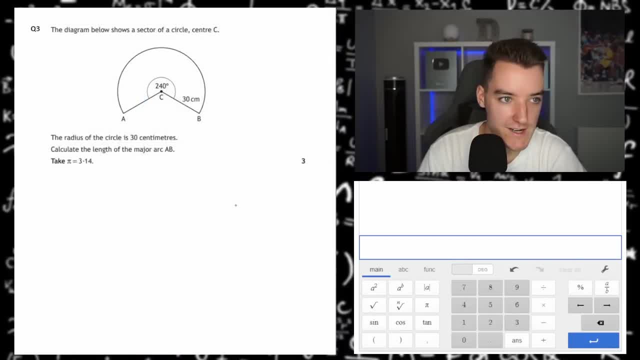 okay, so moving on, question three looks like we have a bit of circles involved in this question, so this one's also non calculator we have. the diagram below shows a sector of a circle with center C. the radius of the circle is 30 centimeters and we're asked. 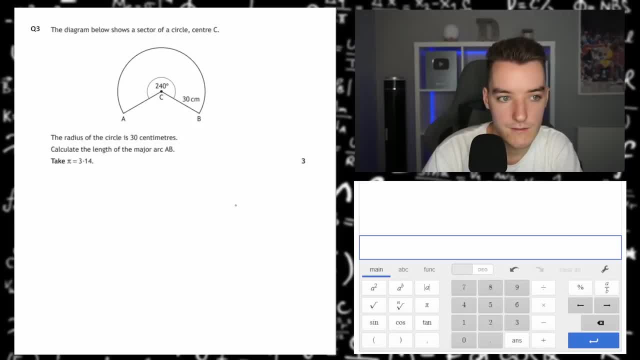 to calculate the length of the major arc. so that would be a to B. so that would be sort of this line here, for those who are confused, what we're trying to work out. we're gonna work out the length of that and we're told to take behind to be. 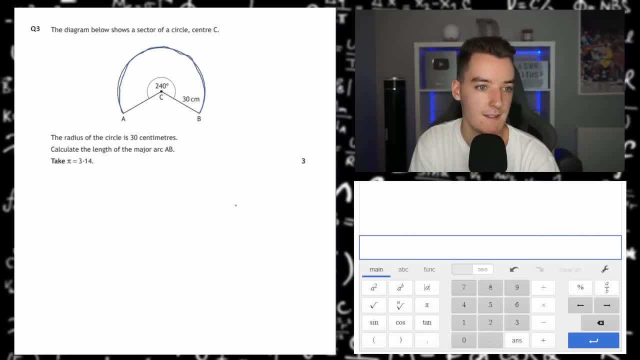 three point one, four. so that is probably why this is alright. well, are we gonna do this? well, pretty straightforward. the circumference our circle is equal to pi D, a fraction of that circumference. We know that AB is going to be a fraction times pi D. Also, D is equal to 2R and R for us is 30.. Pi is 3.14.. Now our fraction is well. 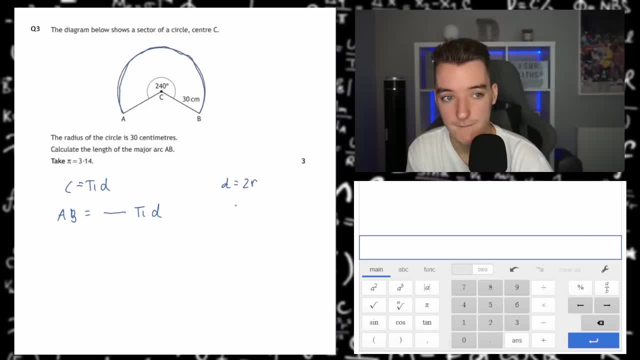 a circle is 360 degrees, so because this arc is 240 degrees of that, it's going to be 240 over 360.. So that becomes, when we simplify it, it's divisible by 120, so it's going to be 2 over 3 times 3.14 times the diameter, which is 2 times 30, which 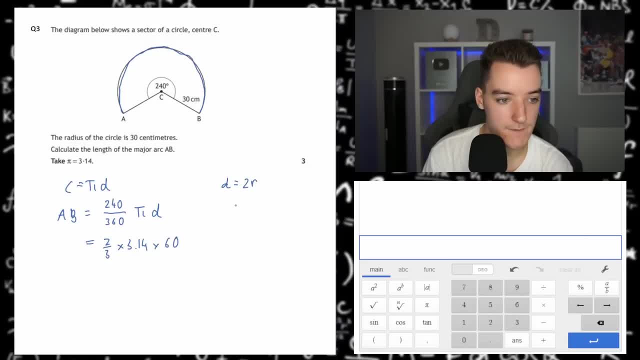 is 3.14 times 3.14 times the diameter, which is 2 times 30,, which is 2 times 30. gives us 60. So all we have to do is work that out, which would be so much nicer with. 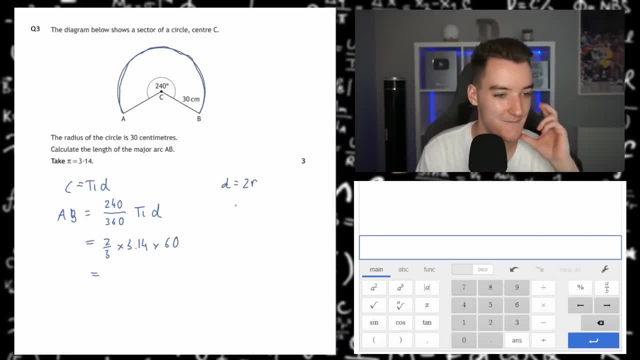 a calculator, but I guess we'll do it. Well, 2 thirds of 60 is 40, so 40 times 3.14.. Well, 10 times 3.14 is 31.4,, timesing that by 4.. That's right, I'm doing a chimney sum get. 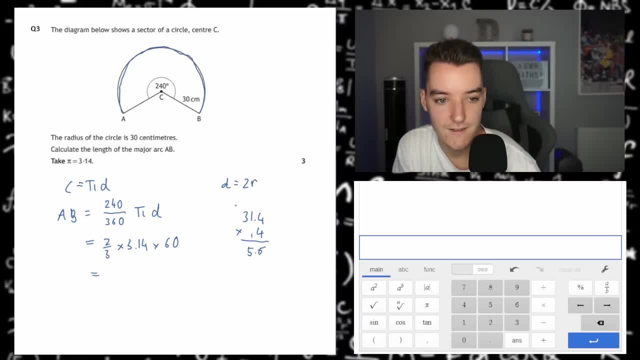 over it. It's going to give us 125.6 centimetres- don't forget our units- And that was not too bad in the end. I really liked that question, Um, and everything looks correct, assuming I've done this right. Hopefully I've not got. 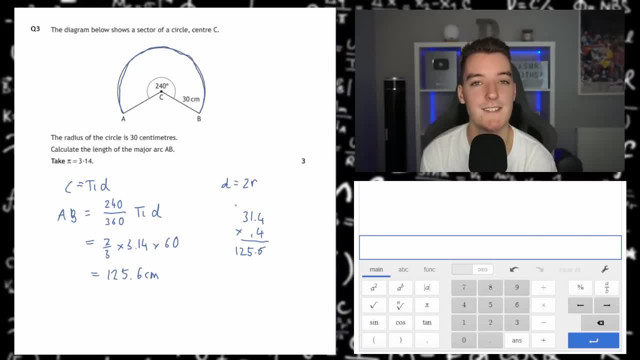 anything wrong, and I'm probably going to get loads of people in the comments screaming at me if I've done any questions wrong, Um, in which case I apologise. If I do make a mistake as I go and I work out when I'm editing, I will pop in the correct solution as I go. 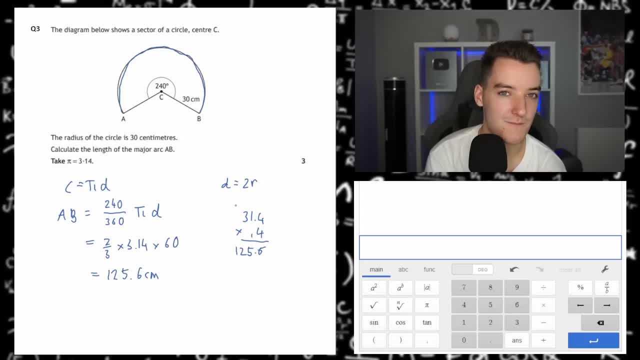 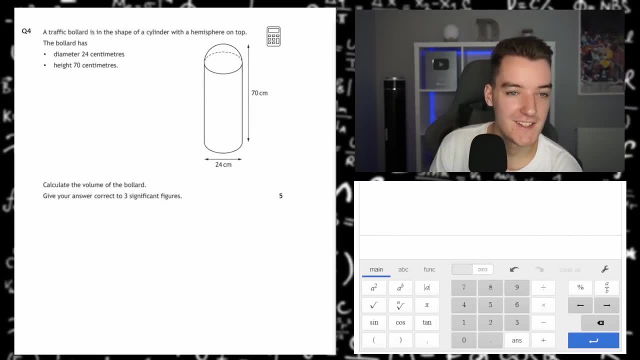 but hopefully, so far so good. Let's go on to question four. Next up we have question four, which eh? finally, we have a calculator question, so we're going to get to make use of my little calculator that I nicely popped down here. 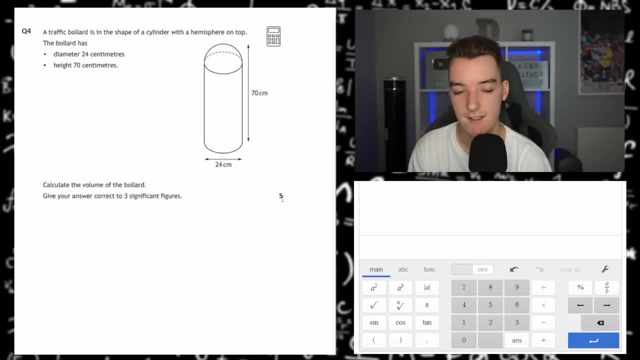 And this one's a big one. this one's five marks, Um, not that we didn't have like five marks in the previous ones, but we'll get over that. Um. so what have we got here? A draft. 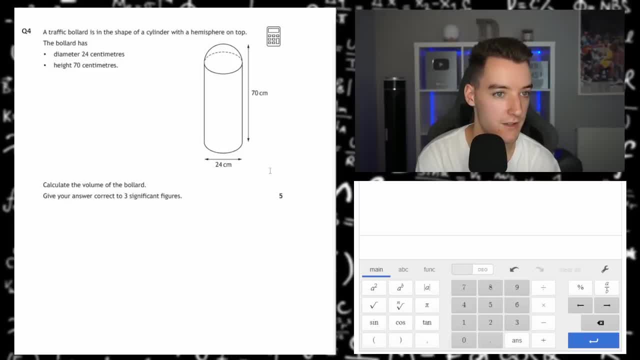 A thick bollard is in the shape of a cylinder with a hemisphere on top. The bollard has diameter 24 centimetres and height 70 centimetres. Calculate the volume of the bollard and give your answer to three significant figures. Okay, so this is why we have a calculator. 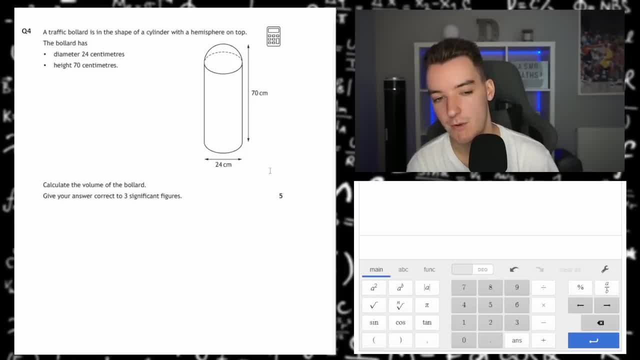 We're going to be working out some volumes Which could get pretty messy. So we have a hemisphere on top of a cylinder and we are actually told the entire height of the bollard. So we're going to have to do a little. 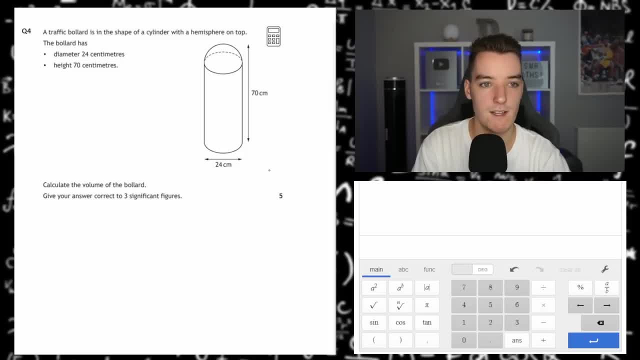 bit of calculating here, because obviously we need to work out the height of the hemisphere. Well, we actually already know that, because we know that the bottom, if you imagine this bit here, this circle that we have here- Um, apologies, that's come up like that: This: 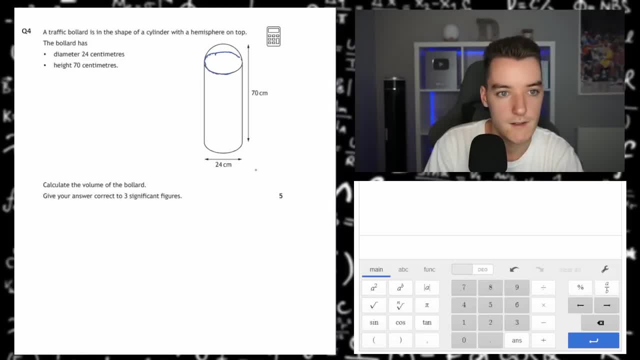 circle is the bottom of the uh cylinder. down here We are. we can see that this is 24 across, So therefore the height is also 24.. Um, so we're going to have to do a little bit of calculating here, because obviously we need to work out the height of the bollard. 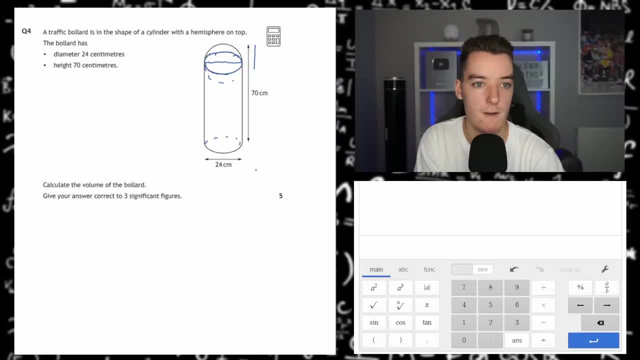 Um, so we're going to have to do a little bit of calculating here, because obviously we need to have to do a little bit of calculating here, because obviously we need to 지금 if it was to continue all the way down as well. However, this is an hemisphere, So it's 12,. 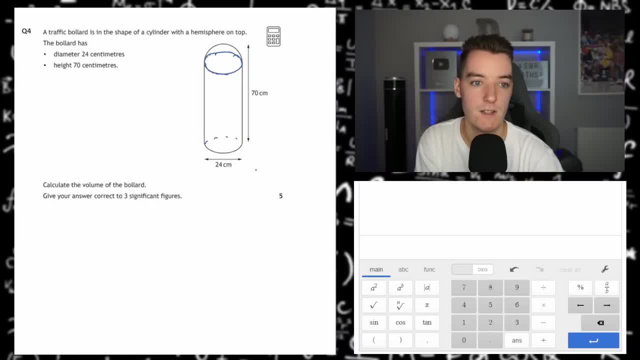 because it's half. So we're going to undo all of this just so we can see the diagram better. So from here to here it's 12 centimeters. I hope that made sense out of there. So if we convert that into a basis, as we always just were ending up with, um, that's 1, 2. 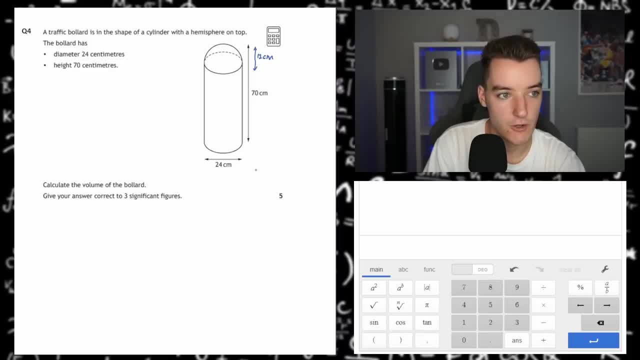 centimeters. So what we're going to have is the volume of the hemisphere. Now the volume of a sphere is 4 over 3 pi r cubed, But this is a hemisphere, So it's 4 over 3 pi r cubed divided by 2.. 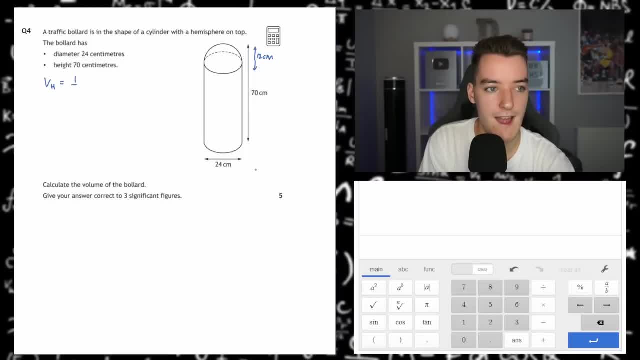 Or we could just say: multiply by a half, So we'd have a half times 4, over 3 times pi, times the radius. Ah well, the radius is just 12 here. Yeah, Cubed, Okay, that's going to be a nasty, nasty number. 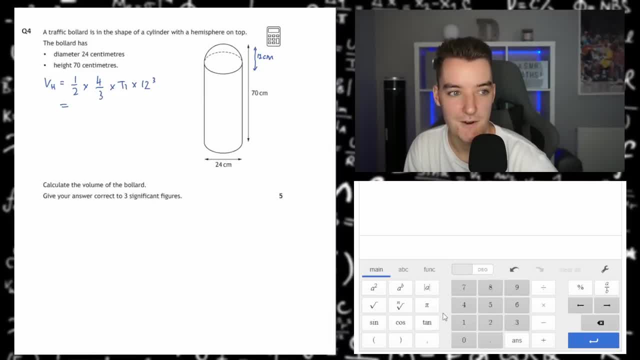 So let's just work that out here. So 0.5 is a half multiplied by 4 over 3.. How can I do a fraction? I'd put it in brackets: 4 divided by 3. Whoops. 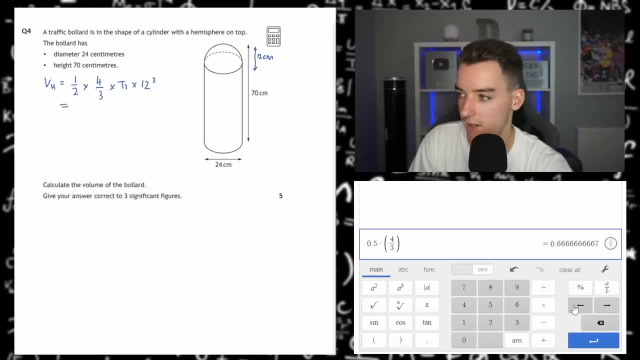 4 over 3.. I'm just making sure you can see all this: A half times 4 over 3 times pi. Is there a pi symbol? There's got to be Pi times 12 cubed Eek, That's not a nice number, but we'll write it in as 3619.114.. 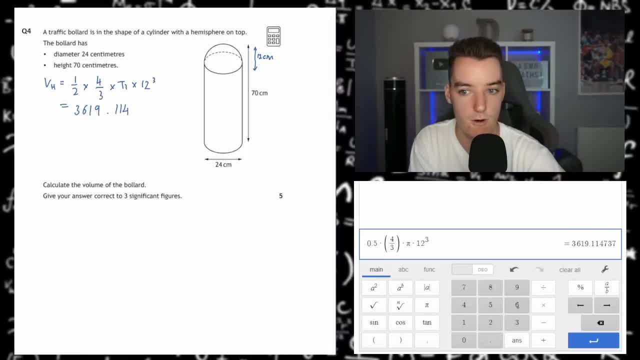 Oh, we'll just write the full thing in. Why not 1147.. 737 centimeters cubed And then next up we have the volume of the cylinder. Now the volume of a cylinder is just the area on the end times, the height. 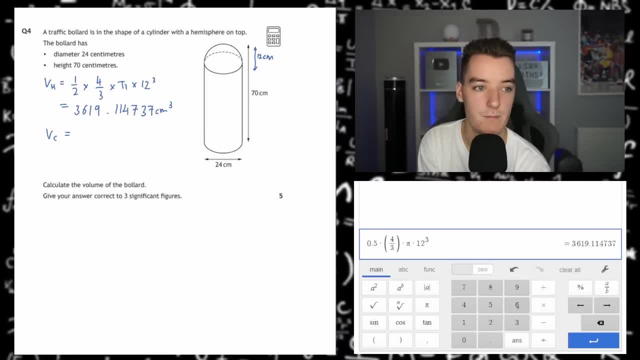 And we all know the area of a circle is just pi r squared. So the area of the cylinder is pi r squared h. So we have pi Times, the radius Times, h. Now the height is 70.. Subtract 12.. 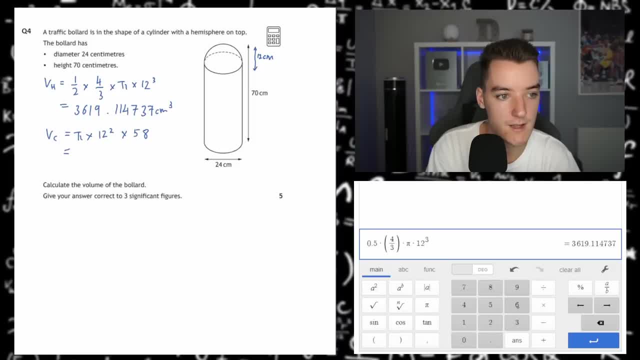 So it's going to be 58.. And the volume of the cylinder is going to give us- Let's just modify this up a bit- Pi r squared, So pi 12 squared Times. First times again, Times 58.. 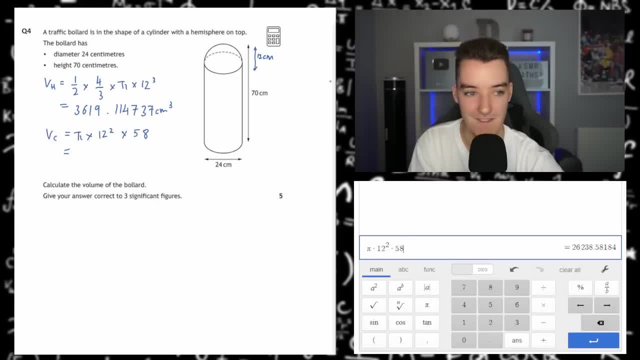 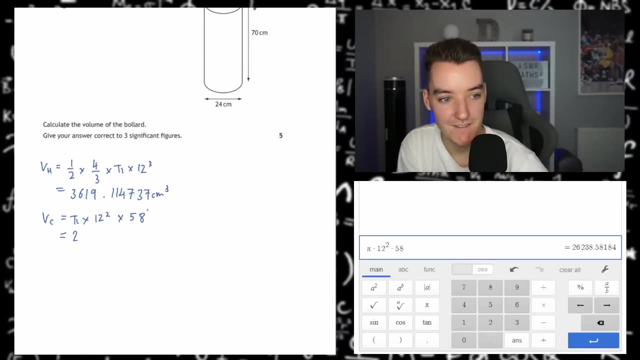 Which is 26,238.. I feel like I was supposed to do this down here. Whoops My bad. 26,238.581.. 1.. 8.. 4 centimeters cubed. Therefore, the volume of the bollard is going to be that plus. 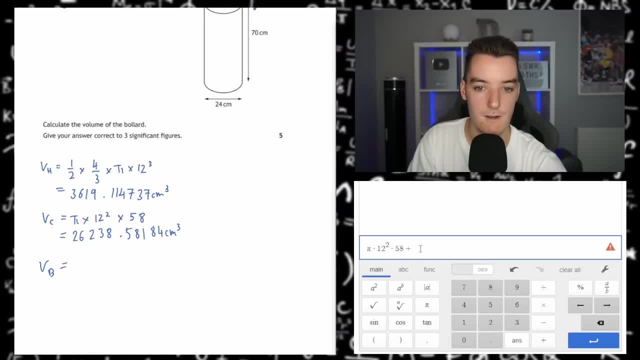 Let's get this actually. Let's copy it. I've never used this calculator, by the way, So it's going to be that plus 3619.. 9. 0.114737.. And then rounding that to three significant figures. 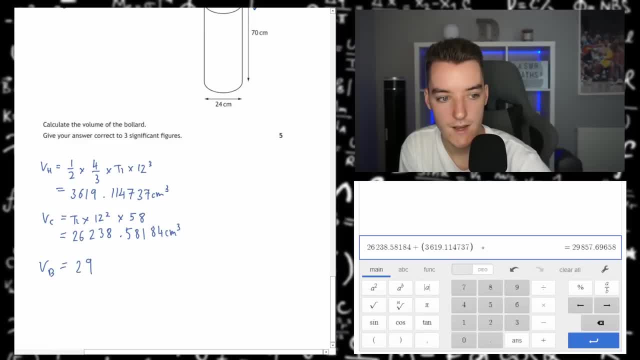 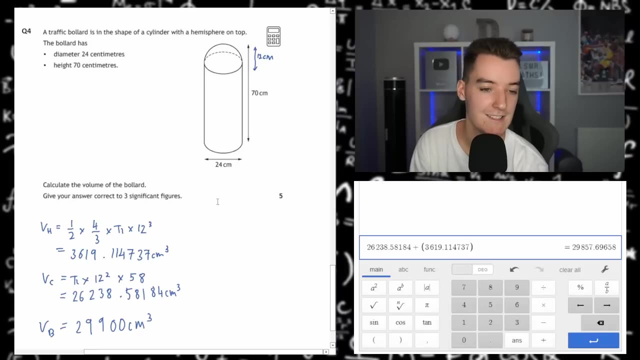 Is 29,900 centimeters cubed. Okay, I think that should be right. That is the volume of our bollard. If we've done that all correct, Five marks- Probably Lots of marks. One for getting the volumes. 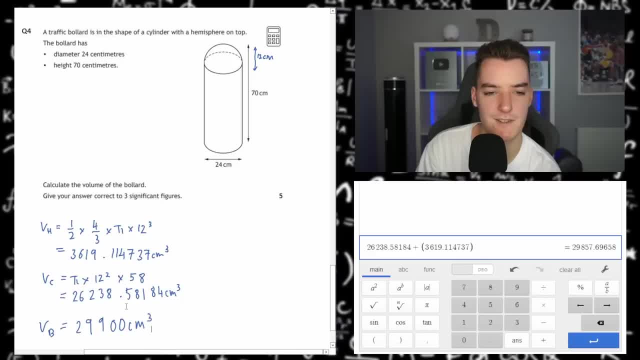 Getting the right formulae And then rounding and the correct answer. It'll all work out somehow. And yeah, Very happy with that question. Let's move on to the next one. Okay, So moving on to question number five. 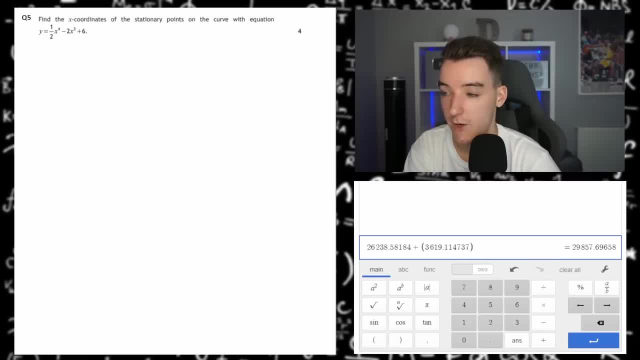 I can't tell if this is going to be an easier question because of how short it is, But we'll see. Question five says The x coordinates of the stationary points on the curve with the equation: y equals half x to the power of four minus two, x cubed plus six. 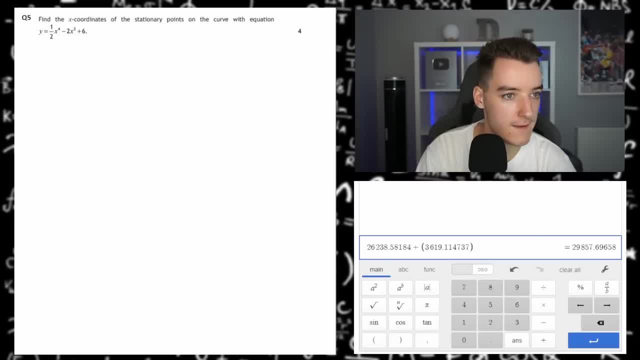 Okay, So stationary points. Well, one thing we know about stationary points is they occur when The derivative dy by dx is equal to zero. So, in other words, we need to derive or differentiate this equation. So for us, dy by dx, differentiating. 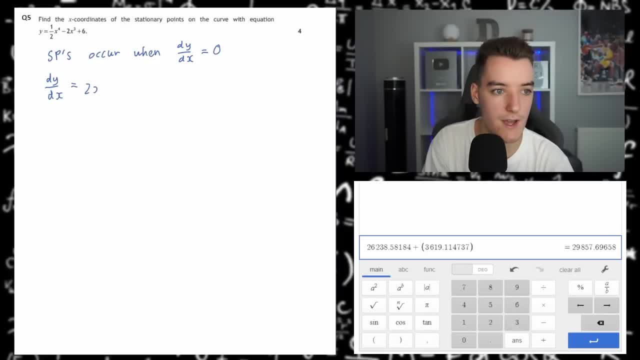 We're going to get four times a half, which is two x And degrees, the power cubed. the next one, we're gonna get minus 6x squared- we're just doing simple differentiation here, by the way- and then the last one is 0 and this is gonna be. 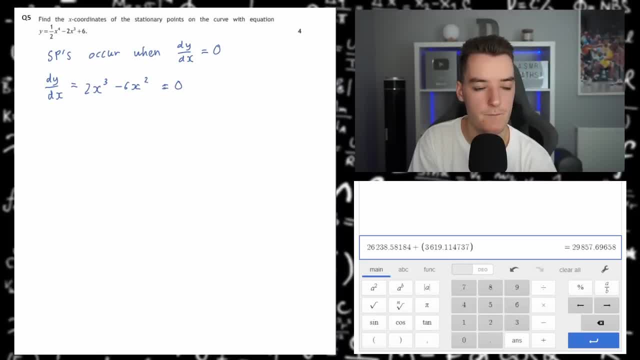 equal to 0, and now we simply want to just factorize here. so to factorize this, we have a common factor of 2x squared multiplied by X minus 3, so we are going to get as our X values. or because this is equal to 0, so we are going to get as: 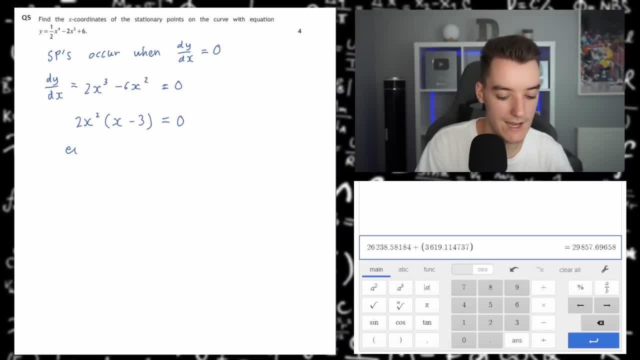 our X values either. well, we'll get two values, so we'll get: X is equal to 0 and X is equal to 0, and X is equal to 0 and X is equal to 3, and that is just to make this on the left- equal 0. you see, if X 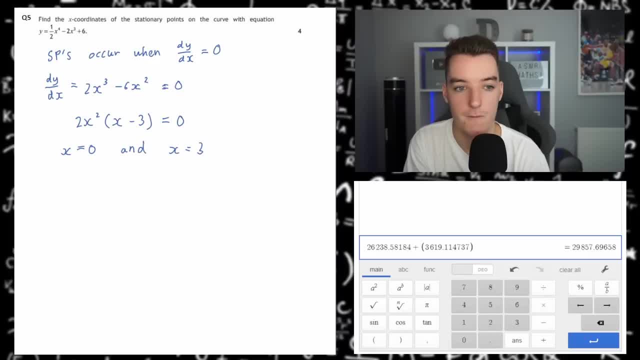 was 0, substitute it in, you get 0. if X was 3, substitute it in, you'll get 0. and actually you know what I'm surprised. that was worth four marks. that was really, really simple. I feel like the question should ask: find the coordinates? 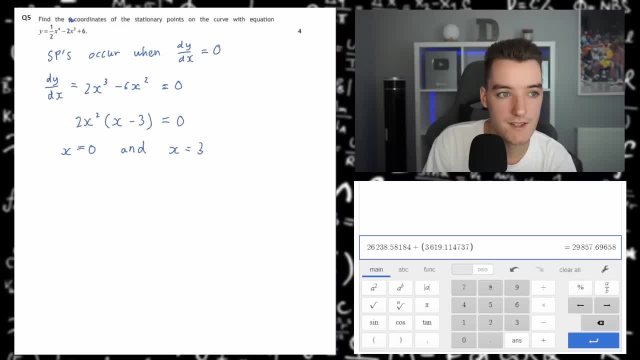 actually I am really mushrooms, which I don't like. I really wanna be strong. it actually scratchy. well, just the X coordinates, because, no, we could technically work out the coordinates and you know what, screw it, I'm gonna do it. let's work them out. so when X. 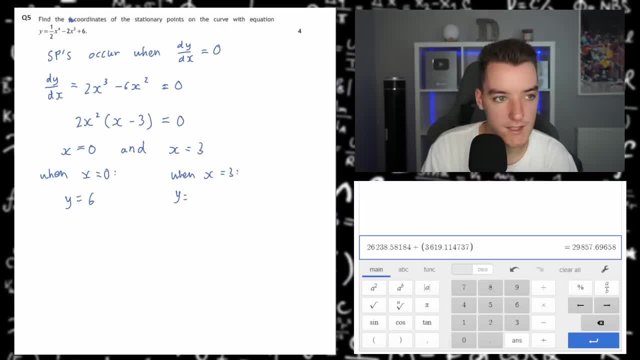 is 0. Y is equal to a half times x to the power of 4.. 3 to the power of 4,. well, 3 cubed is 27.. So 27 times 3 is 81. So 81 multiplied by a half is 40.5.. 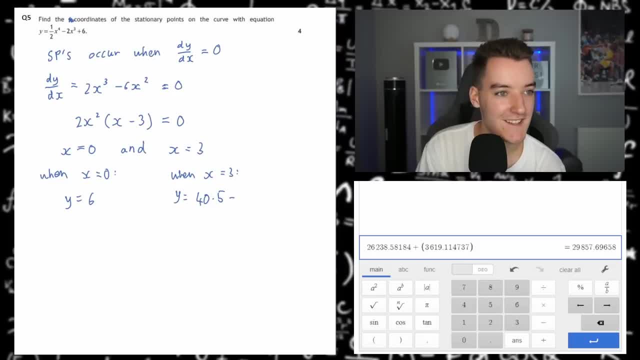 I probably shouldn't be doing this. Subtract 2 times 27,, which is 54, plus 6.. So y is going to be 40.5,. take away 54,, which is minus 13.5, plus 6 is minus 7.5. 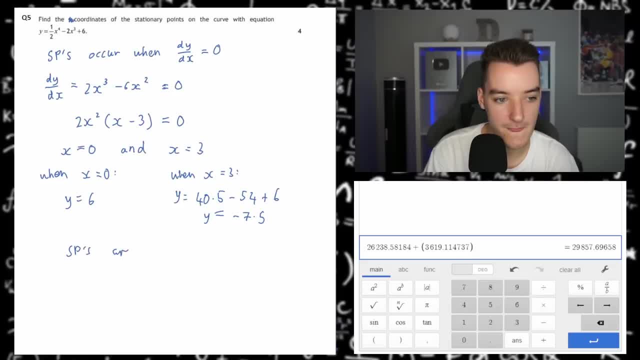 So the stationary points are 0,, 6, and 3, minus 7.5.. I may have messed up that second one. I've just done it really quickly. Someone can check it for me, Let me know. But I know that's not what we're meant to do. 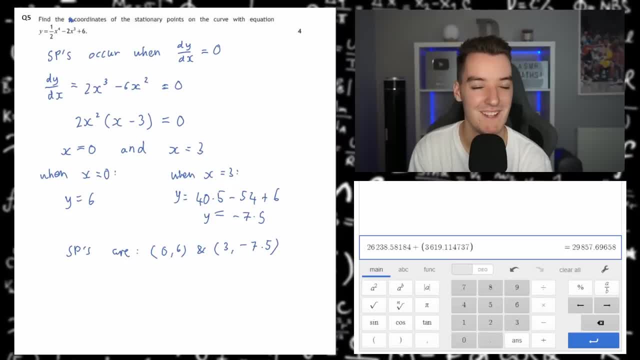 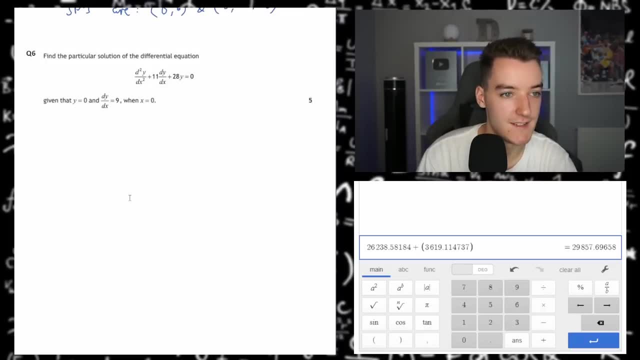 but do I get an extra mark? Maybe Let's go on to question 6.. Okay, so question number 6 is a bit of a juicy question. actually, We are asked to find the particular solution of a differential equation which we can see right there. 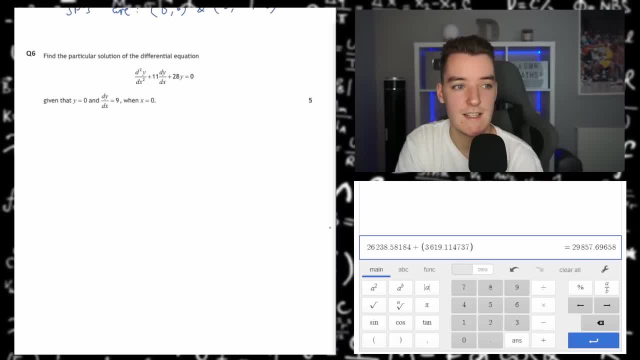 And we've got the initial conditions Given, that y equals 0, and the derivative of y equals 9, when x equals 0. Okay, well, for those who don't know much about differential equations, the first step to do when solving them or finding a particular solution. 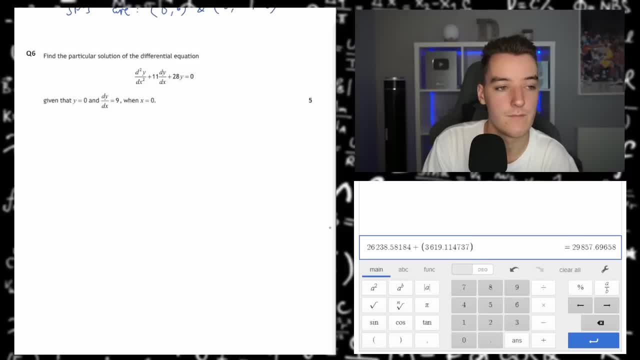 is to find the general solution, And the first step to finding the general solution is solving what is called the auxiliary Equation. Now, our auxiliary equation is going to be k squared plus 11k plus 28, equals 0.. 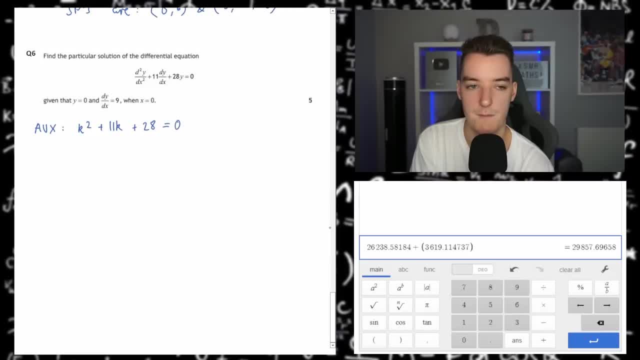 It's quite lucky that it's equals 0.. It's not going to make things too difficult. So when factorizing this, nice and easy k plus 7,, k plus 4, so therefore k equals minus 7, or minus 4.. 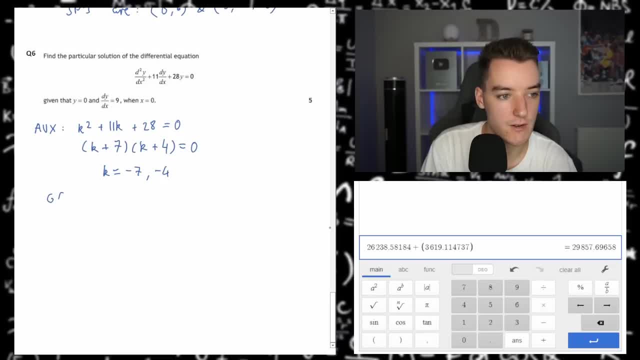 So we have our values for k. Therefore our general solution, if I remember, is: y is a equal to ae to the minus. oh, no to the first k1, plus be to the k2, I think. So in our case it's going to be: y equals ae to the minus 7,. 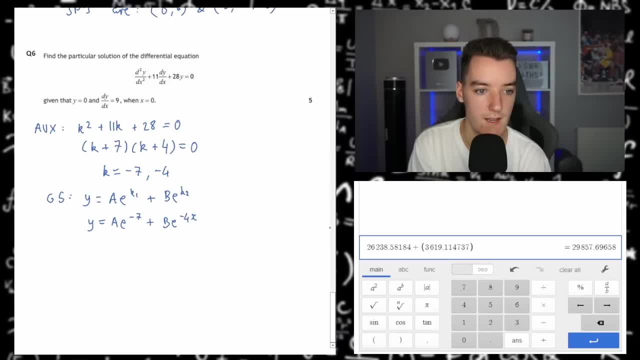 plus be to the minus 4, oh, forgetting the x. I think I think that's right. It's been a while since I've done this. I'm not going to lie to you all. So that's our general solution. 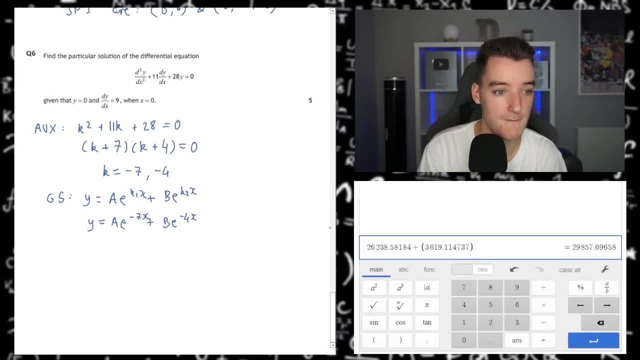 Now to find the particular solution. Well, when y is 0, or y is 0, when x is 0. So y of 0 gives us 0 is equal to ae, and because x is 0, this is going to be just 1.. 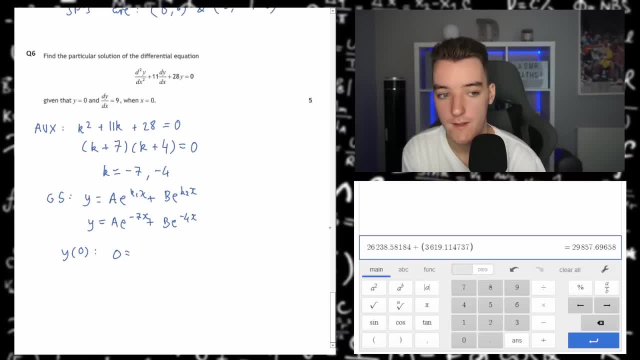 Because anything to the power of 0 is 1.. So we get 1 times ae, which is ae, And then the same for this second one. So we get ae plus be is equal to 0.. It's the first equation that we're going to be using. 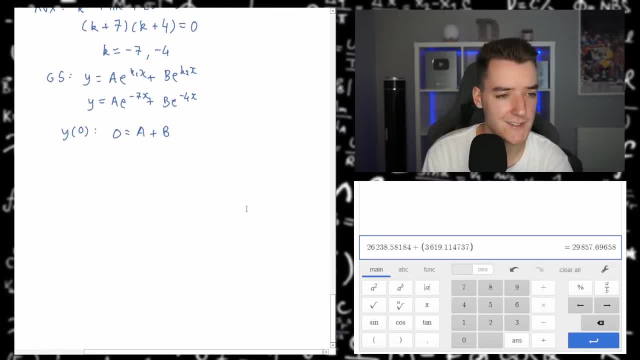 Looks like we're going to be doing a bit of simultaneous equations. And then for the second one, well, we need to differentiate, because we're told the derivative is equal to 9.. So let's differentiate and find dy, dx. So differentiating gives us minus 7 ae to the minus 7 x. 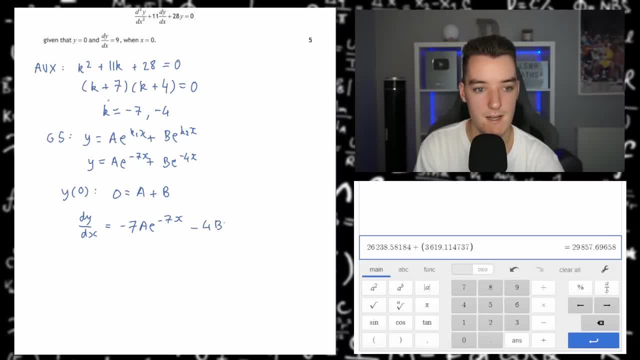 Minus 4 be to the minus 4 x. This is just simple differentiation. And then dy by dx. Um, Sorry, this here Y is 0.. If I had like written this wrong, I feel like it should be x of 0.. 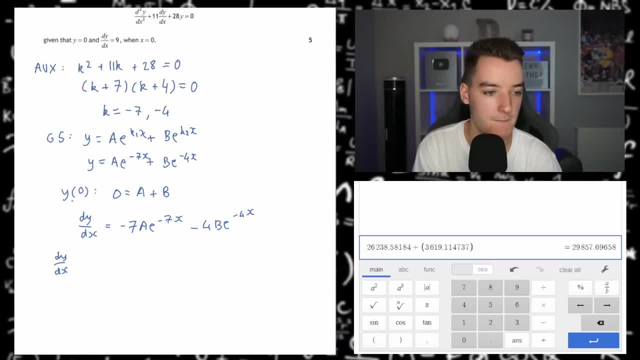 Ah well, I've probably written that wrong, but I know what it means. Um So 9.. Yeah, I definitely have. But what I'm basically saying is: 9 is equal to You. just input x of 0.. 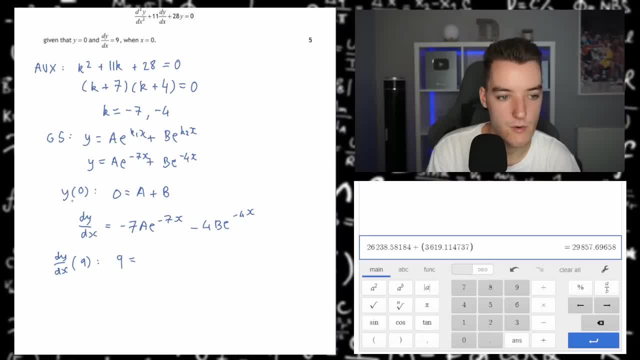 Um, So we're going to have minus 7 a, minus 4 b, And these are our two equations that we're going to use to solve for a and b. So let's solve for a and b here. Well, we can rewrite these. 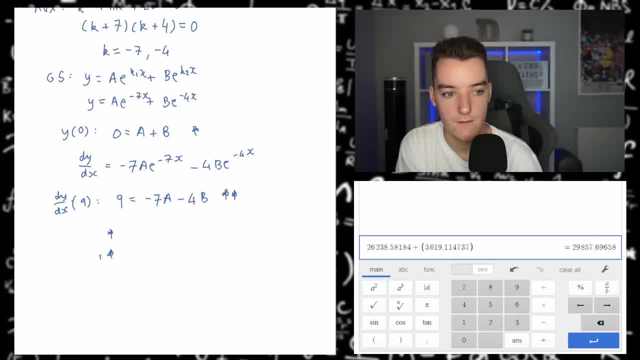 Um, I'm just going to double star this one. Let's multiply the top equation by 4. And we're going to get 4 a plus 4 b equals 0.. Minus 7 a, minus 4 b is equal to 9.. 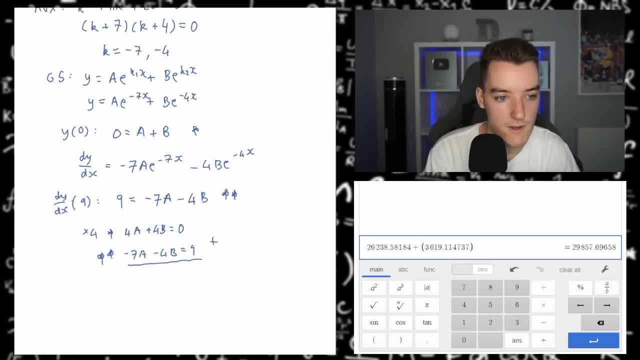 Add these guys together And once we've done this, we're going to get 4 minus 7 is minus, 3 is equal to 9.. Uh, minus 3, a, sorry, So a is going to equal 3.. 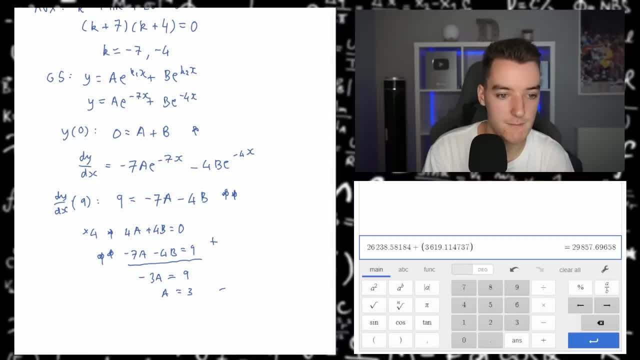 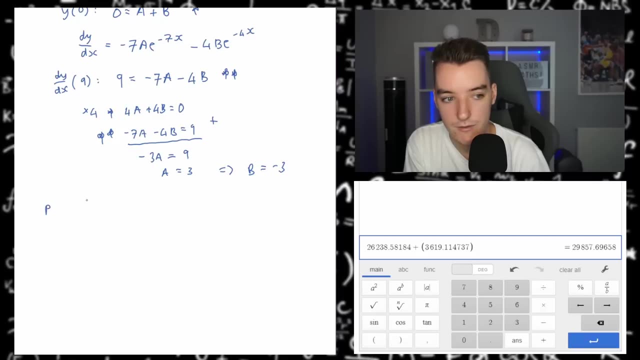 Input that into the first one. Well, we're just going to simply get that b is equal to minus 3. And that should be pretty nice. So now, once we've found these, we can officially work out our particular solution. 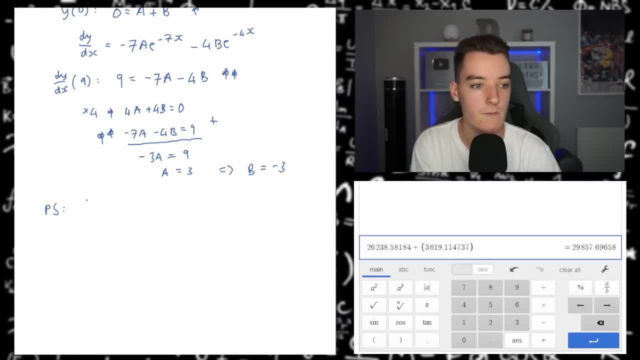 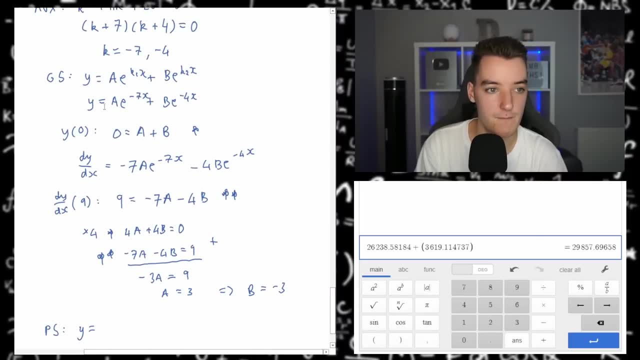 Particular solution. So our particular solution is going to be: y equals. So our general solution. but substitute a and b is what we've worked them out to be. So a is 3 e to the minus 7 x, plus b, which is minus 3 e to the minus 4 x. 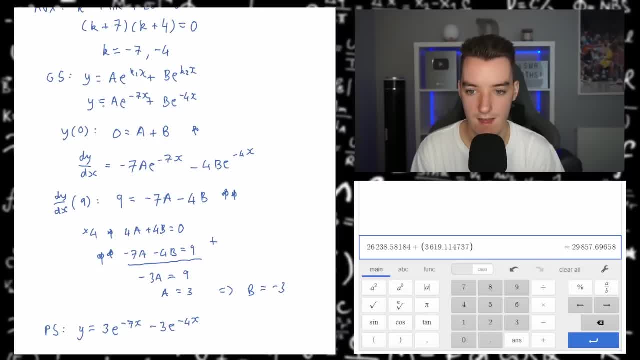 And that is that. It's been a long time since I've done these questions, So I hope I've done that right. Also, I forgot to clear my calculator, but it doesn't matter And that was a lot of fun. 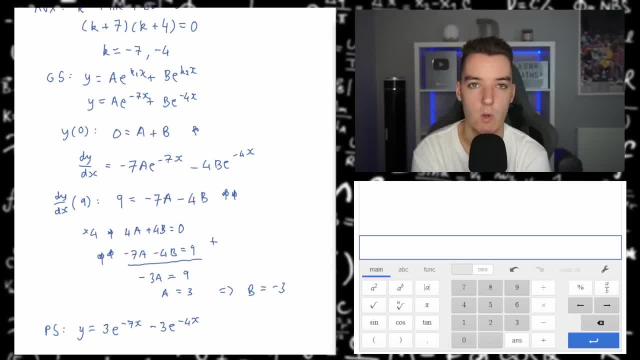 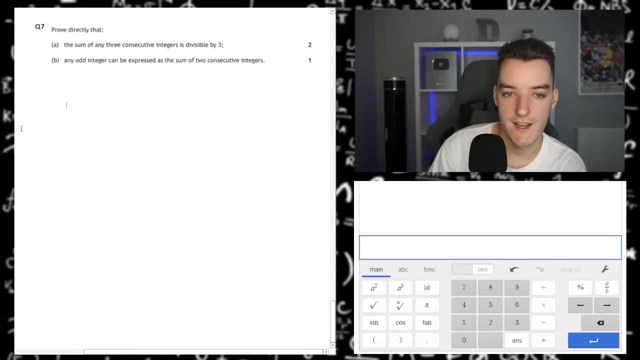 A little bit of a sort of memory test, because it's been so long since I've done questions like them. But nice, That was a lot of fun. Okay, question number 7.. Question says: prove directly that First part: the sum of any three consecutive integers is divisible by 3.. 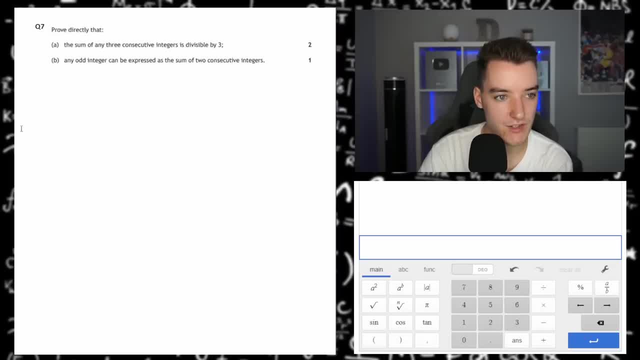 And then part b. any odd integer can be expressed as the sum of two consecutive integers. Okay, I love direct proofs, Especially when they're literally two and one marks. That means it's going to be very easy, Very, very easy. 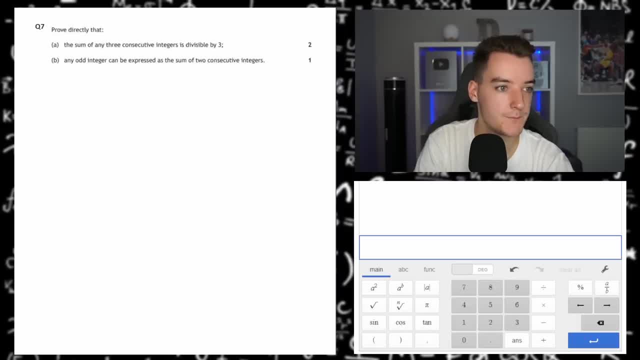 So let's give this a bit of a go here. So part a: The sum of any three consecutive integers. Well, let's take three integers as k. The next one is k plus 1.. So k plus 1.. 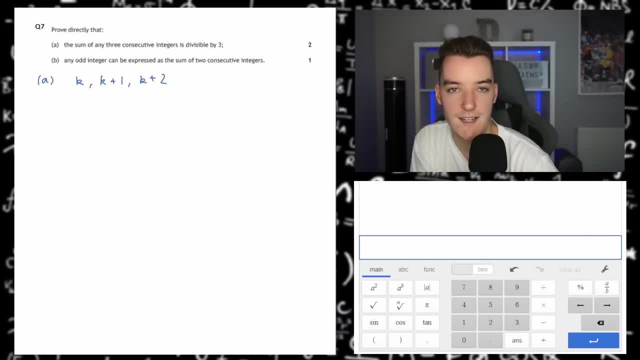 And the next one is k plus 2.. That's three consecutive integers, right Where the integer is k. So we'll say that k is in the integers. Then we want to work out the sum of them. So the sum of these is k plus. 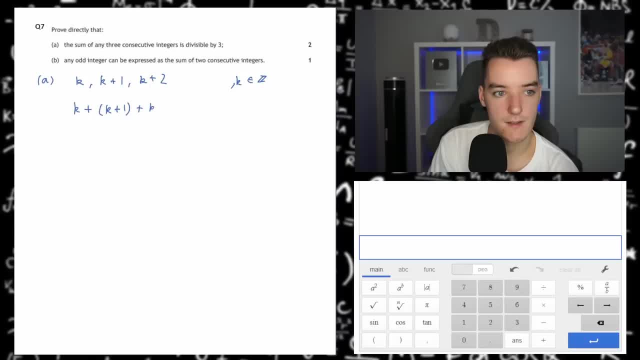 k plus 1 plus k plus 2.. And this is equal to Well, we can see 3k plus 3.. Which, well, when we It's obvious, it's divisible by 3.. But what we've got to do is take out the factor of 3.. 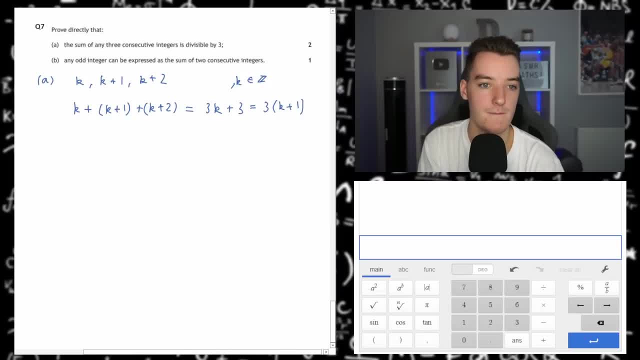 And we get k plus 1.. And we would just say sort of Which is divisible by 3.. And this is simply because, no matter what this is, Whatever value k is Multiplying it by 3 or dividing it by 3.. 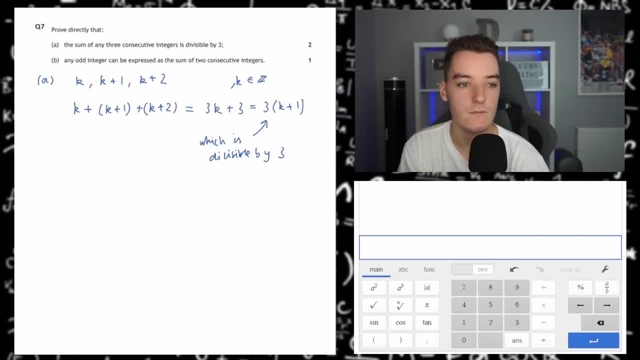 We're going to get that basically. So that was good. Let's do part b, Which says any odd integer can be expressed as the sum of p, The sum of 2 consecutive integers. Okay, So 2 consecutive integers. 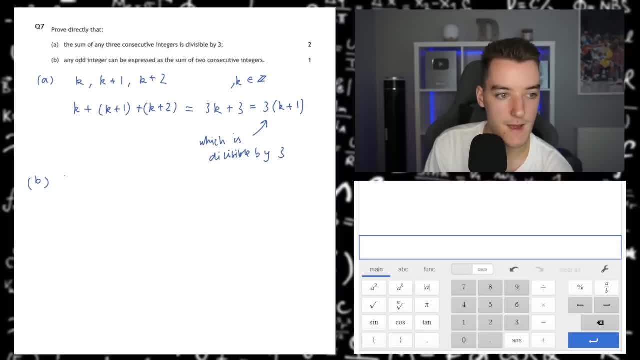 Again, let's take this time- m And m plus 1.. There are 2 consecutive integers Where m is an integer. Any odd integer can be expressed as the sum of 2 consecutive integers. Any odd integer can be expressed as the sum of 2 consecutive integers. 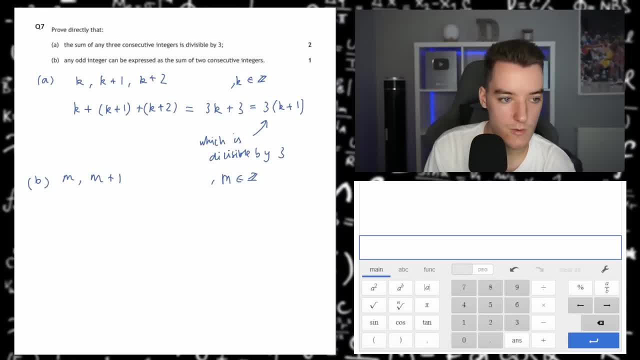 integers. Okay, so let's just show that m plus m plus 1 is equal to 2m plus 1, and this is clearly odd. Which is odd? And the reason it's odd is because if you take any integer m, multiply it by 2, you get an even integer. So if you add 1 to an, 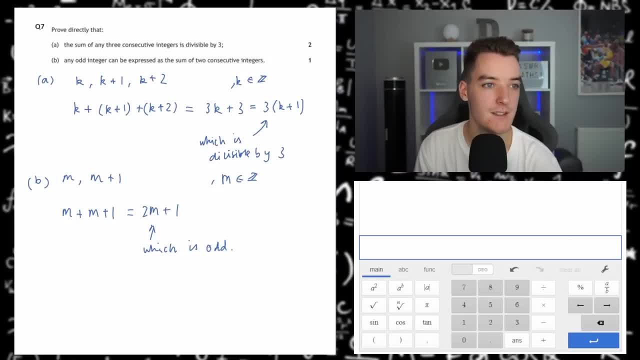 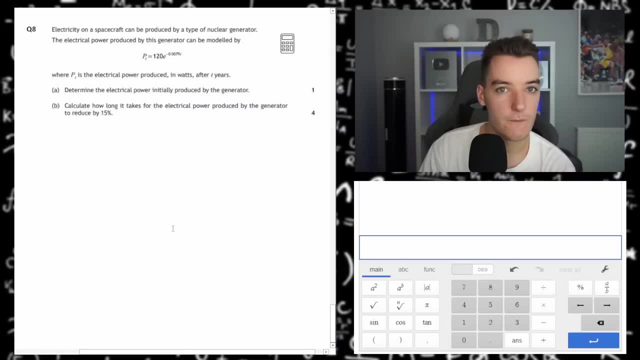 even number. you're gonna get an odd number. So that was super, super easy. question done. No calculator even needed. For question 8, we are going to be allowed to use our calculator again. Yay, It's not gonna be just Sather doing. 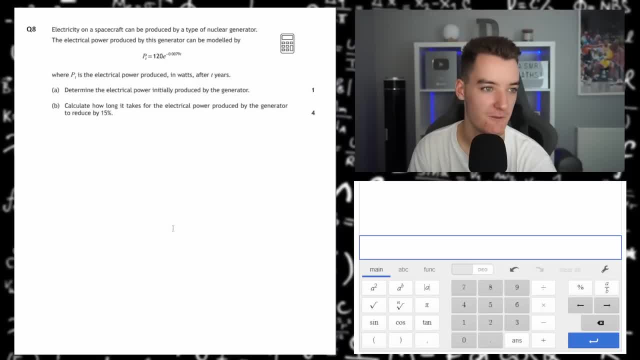 nothing again. Let's actually take a look at the question first, though, before we get too excited. Electricity on a spacecraft- oh, this sounds interesting- can be produced by a type of nuclear generator, The electrical powered. the electrical power produced by this generator can be modelled by the amount of power produced at any time. d is equal. 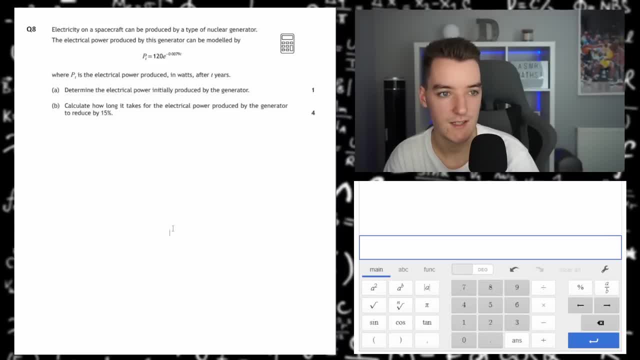 to 120e to the power of minus 0. point might be hard for you guys to read, but minus 0.0079 d, Where bt is the electrical power produced in watts after d years. Part 1 says: determine the electrical power initially. 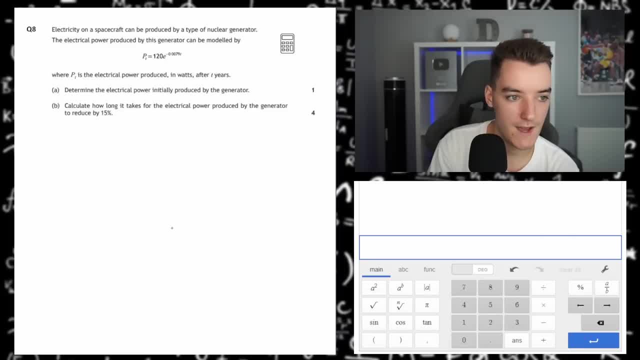 produced by the generator. Well, that is literally the easiest question we'll get in this paper. So initially, at time equals 0, pt is 120e to the power of 0.0079 times n. what that's gonna give us is zero, and I said earlier, anything to the power of zero, just gives 1.. So eat, the power of zero is 1.. 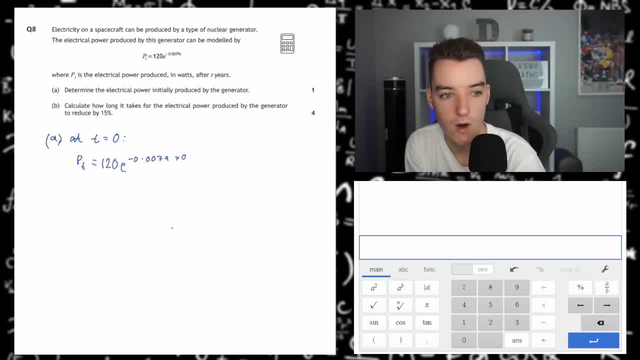 well, I said earlier, anything to the power of zero, just gets one. so eat, the power of zero is one gives 1.. So E to the power of 0 is 1 times 120.. Initially it's 120 watts, which is actually the symbol W. Alrighty, let's move on to part B, which says calculate how long it takes. 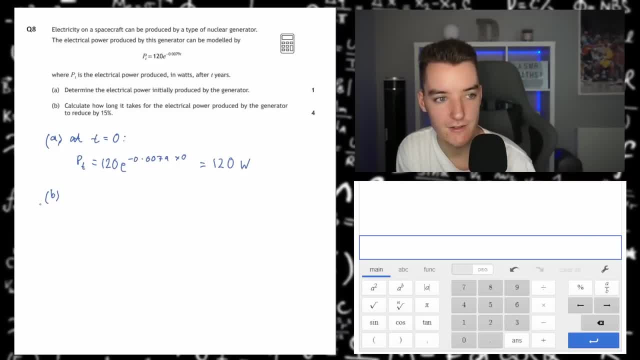 for the electrical power produced by the generator to reduce by 15%. Okay, so what we want to do is work out how long it is. So we're trying to work out D And after the power by the generator has reduced by 15%, so if it starts at 120, we want to work out how long it takes. 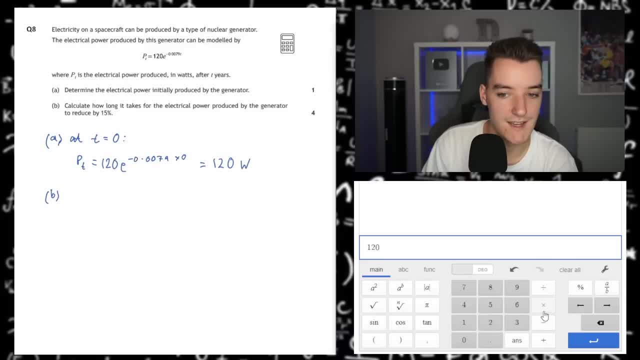 to get to 15% less than that, Which is 102.. So we have: 102 is equal to 120 E to the minus 0.0079 T. Okay, good start, But what we're trying to do now is take what we have here and work out what T is. 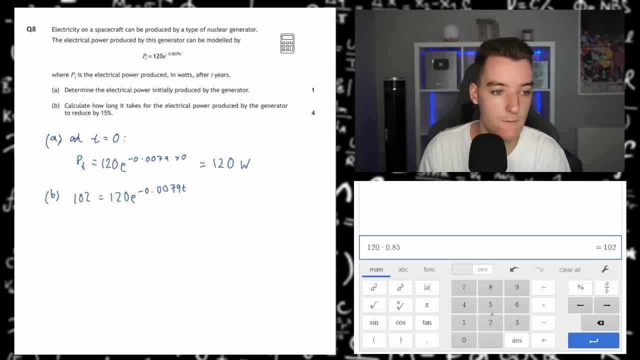 And to do that well, first things first, let's get rid of this 120.. So let's divide both sides by 120.. So 102 divided by 120 is, funnily enough, 0.85.. Should have known that. 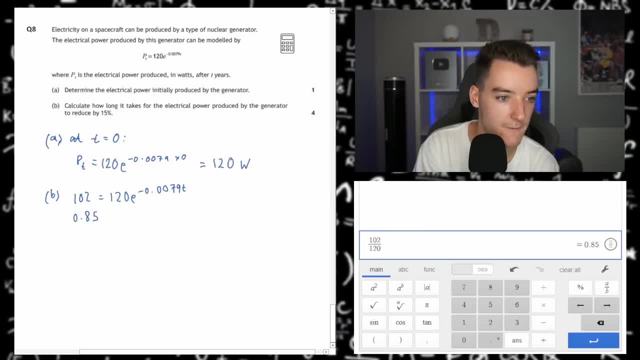 to be honest. So 0.85 is equal to E, Exponential, Exponential 0.0079 T. And to get T on its own, all we want to do is take the logarithm base E of both sides. Now, sometimes we just call that LN. I'm going to call it LN, It's called the. 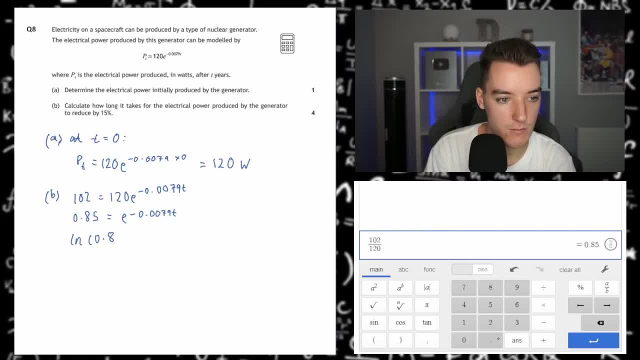 natural log, So the natural log of 0.85.. When we do that to the other side, because we're taking the natural log of E, that just cancels out, So we're going to just get negative 0.. Will it give us a negative, though? I think so Yeah, negative 0.0079 T, And so to work. 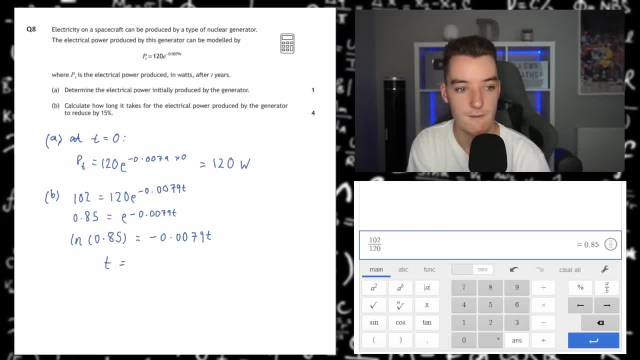 out T. all we want to do, 0.0079 T, Is divide the natural log of 0.85 by negative 0.0079.. So let's do that. I don't know what that I didn't mean to do that. Okay. so natural log: Where is that? 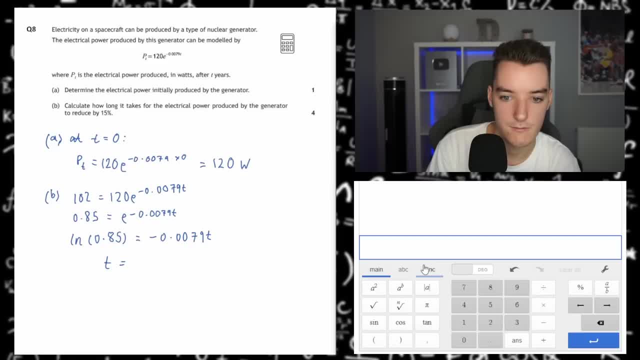 We're going to need a fraction eventually, So is it in here. LN, LN, there we go. LN of 0.85 divided by minus 0.0079 gives us- that seems to be right- 20.57, roughly. 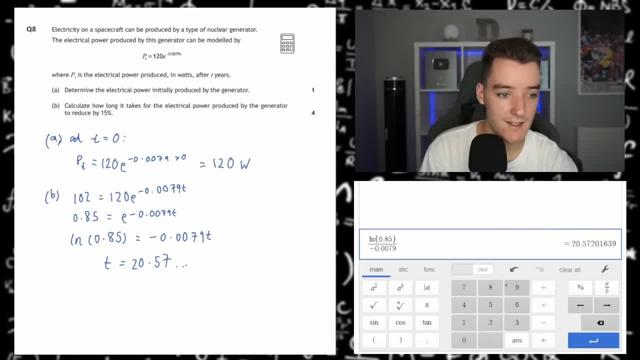 Okay, So it's going to take approximately 20 and a half years. I think it said it was in years, right, Yep? So 20 and a half years approximately for the power to reduce by 15%. There we go. Very nice question. 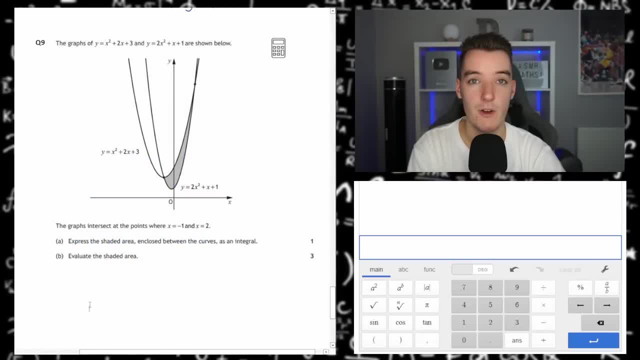 On to question nine. All righty next up Looks like we have a little bit of an integration question and it's calculator as well, So looks good, Let's. I love the diagram on this as well, So let's have a little look at what we're working with. So we have the 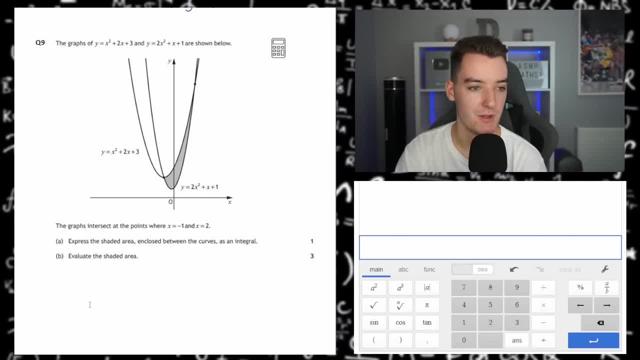 graphs of those two curves are shown below, below, below. The graphs intersect at the points where x is one and x is two. Express the shaded area enclosed between the curves as an integral. Okay, so what? we all know that the area between two curves is just the. 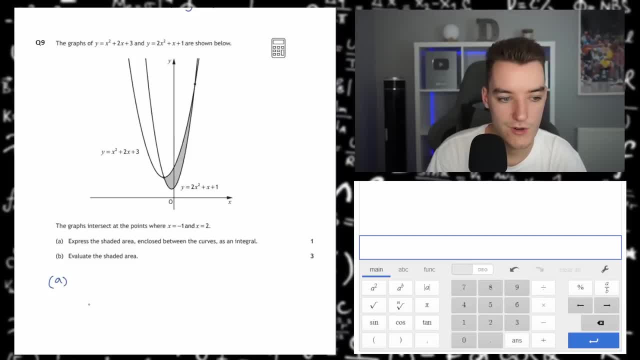 integral of the top curve. Subtract the bottom curve, And then the limits are where those curves cross. So the limits are minus one and two, or the boundaries if you will, And it's going to be the top curve, which is x squared plus two, x plus three. Subtract the. 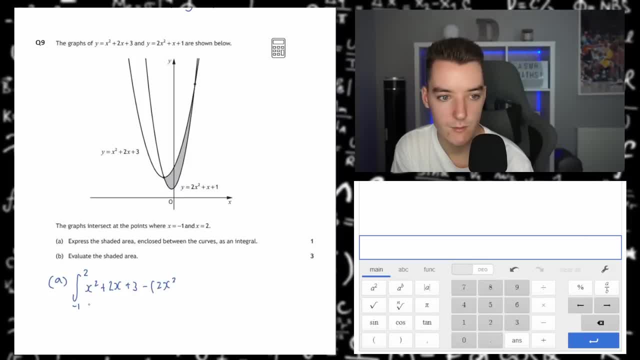 bottom curve Minus two x squared. It's going to be minus x, but we'll keep it as plus because I'm doing extra working here, And then that is simply going to equal minus one to two of minus x squared. Let's put the bracket around this. 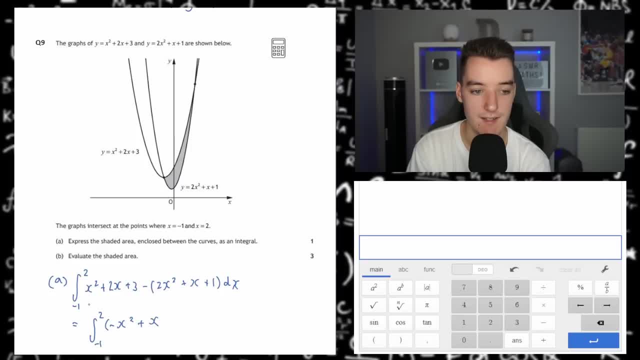 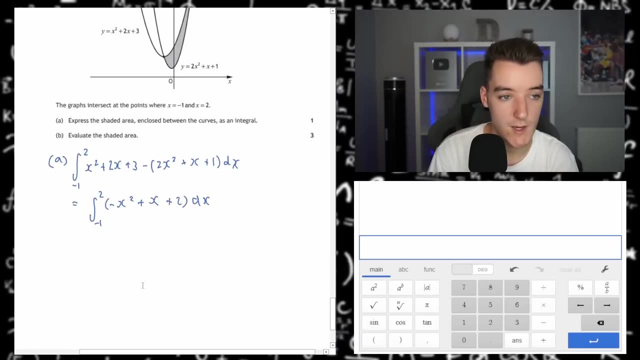 So plus x, plus two dx, And that is that. So that's very nice. That is the integral, And part b just simply asks us to evaluate the shaded area. So what we're going to have to do, to start with, is, well, integrate the integral, And then, because we're allowed a calculator, 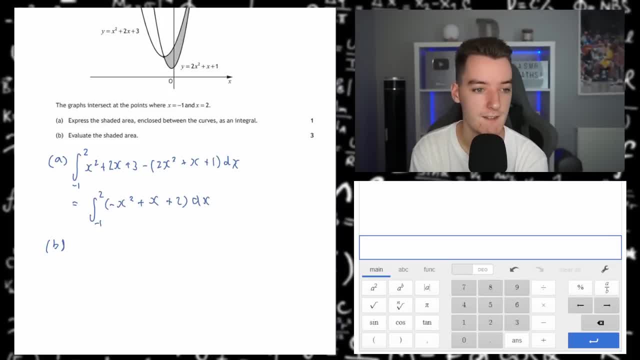 substitute in the limits. So evaluating the integral Minus x squared, integrated is just minus one third x cubed x integrated is plus one over two x squared And then two integrated is two x And we are evaluating it. I like to do little square boxes. Some people do. 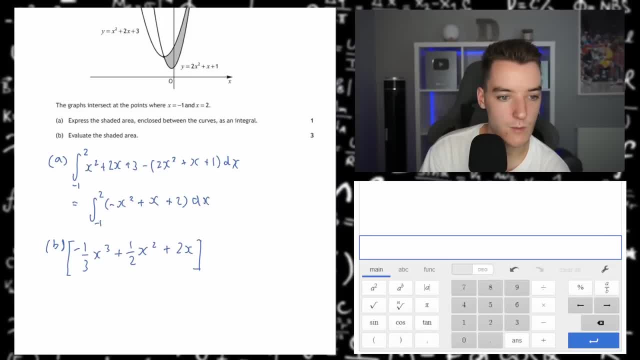 just a straight line. Add the values where x is equal to two and x is equal to one. So let's substitute that in And I won't do any working. I'll just do this all on the calculator because I'm lazy. So, substituting in the first one, we're going to have minus one divided by three multiplied. 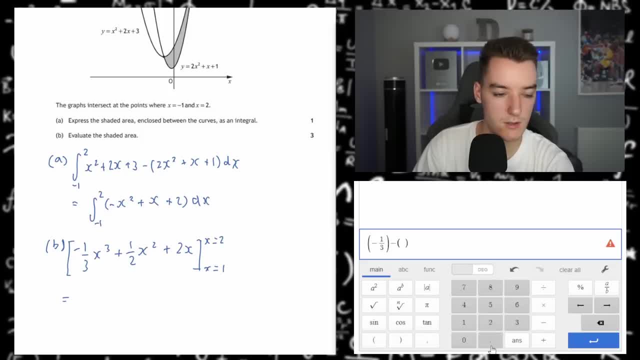 by Two cubed. Let's put it up here: Two cubed is just eight. Wait, why did I do a point? There we go, Then we're going to have plus one divided by two, And then that's going to be multiplied by two squared. 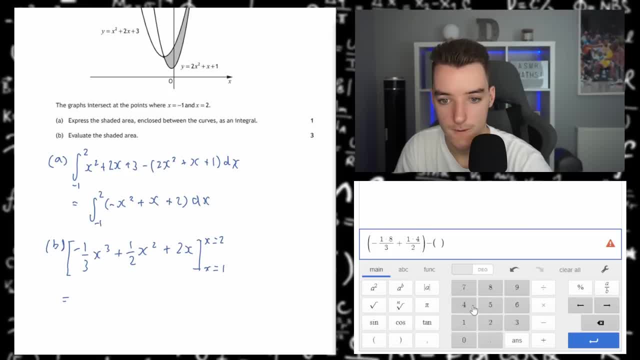 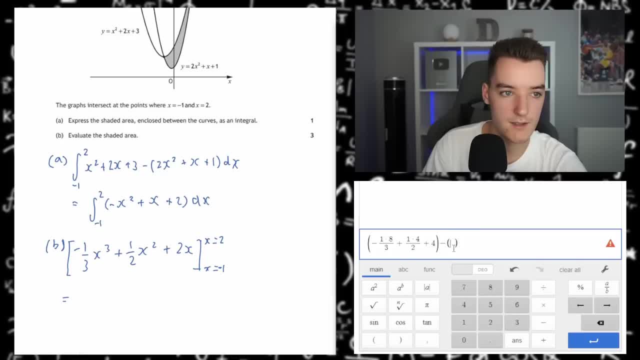 My bad. Substituting negative one is going to give us again negative one divided by three. So we'll simply multiply it by negative one, cubed, which is just negative one, And then plus a half times one, And then plus two times negative one, which is minus two, which. 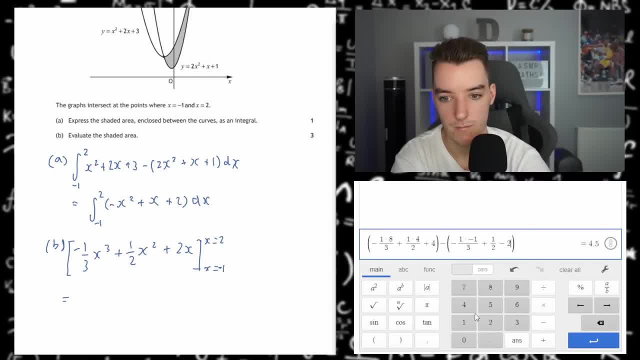 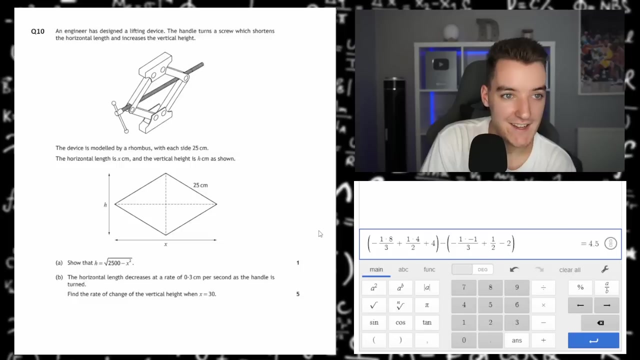 gives us four, four, point five, which is just nine over two. right, that should be right. that should be our area, whatever it is, units squared, I think if I've done that all correctly, everything looks good to me. so, fingers crossed, we've done that right. there we go. that question is complete, okay, so question number ten: things seem. 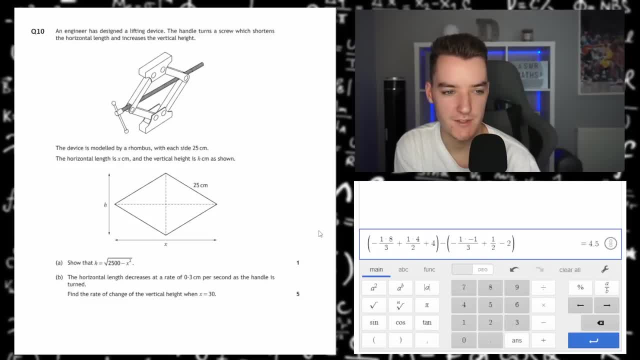 to be getting a little bit cool in this question. maybe looks like a little bit of maybe mechanics or something like that, I'm not too sure. in a way, let's tackle it and see how we get on. so an engineer has designed a lifting device. the handle turns a screw which shortens the 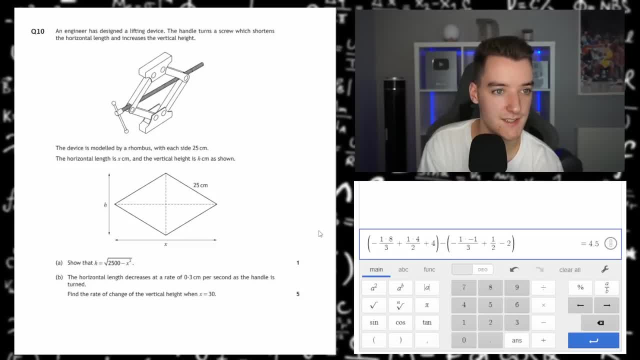 horizontal line length and increases the vertical height. okay, the device is modeled by a rhombus, with each side 25 centimeters. okay, the horizontal length is X and the vertical is H, as shown. show that H is equal to the square root of 2500 minus X. 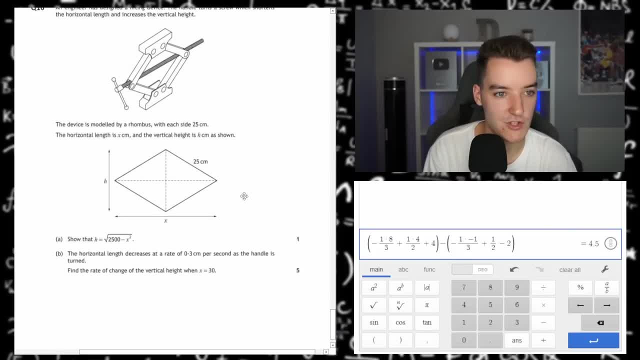 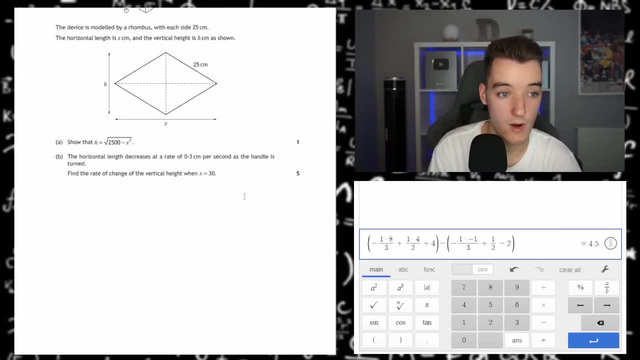 squared, okay, so we're trying to work out H with this diagram, basically. okay, that's only one mark, right? well, the way I would do this is: we can see, we can make these little triangles. they've kind of done that to make it easier for us, so I'm gonna sort of shade it in. oh gosh, my hand is really. 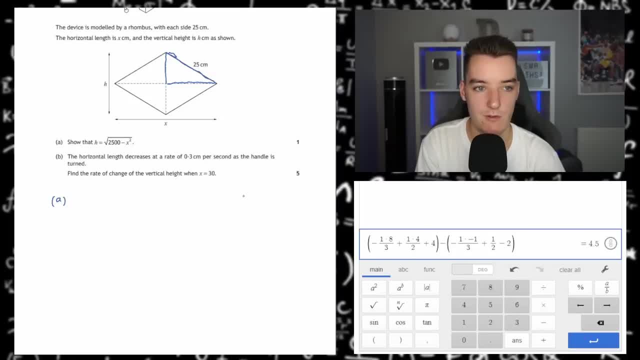 shaky. I will make this triangle well. this bottom side is X divided by two. this side is H divided by two. so, using Pythagoras' theorem, we have H divided by two squared plus X divided by two squared is equal to 25 squared. oh, this one's also. 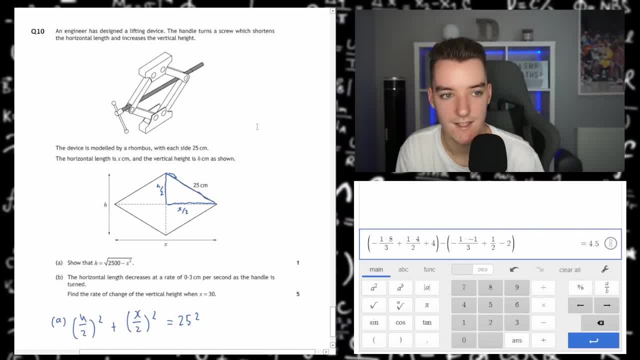 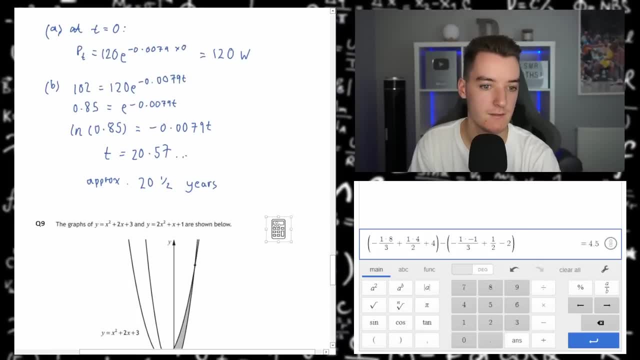 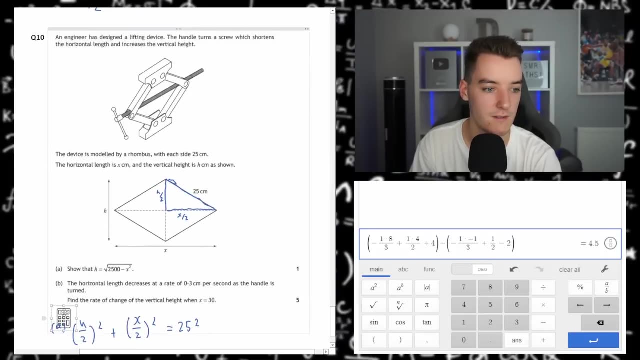 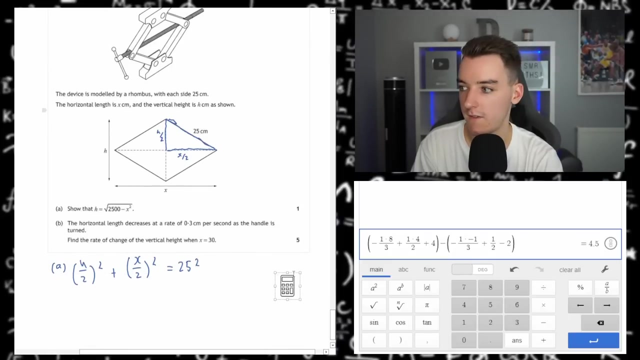 calculator. I know there's not a symbol, but this one's calculated. that's not a later. You know what I'll do? just to be complete, I'll pop in the little calculator symbol right here for us, Just up. Where can I put it? Let's just put it there, That'll do We know. 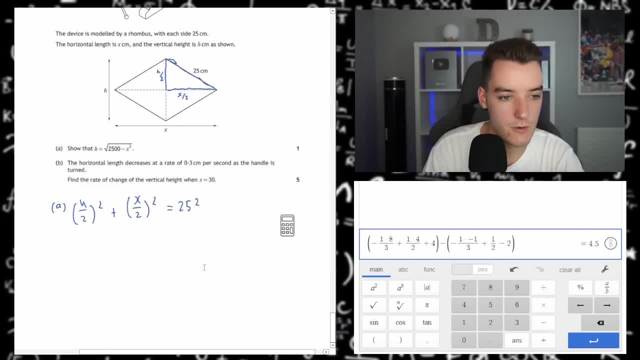 it's a calculator, So we're wanting to find h from this. Well, let's do this. We're going to get h squared over 4, because 2 squared is 4 plus x squared over 4 is equal to what is 25 squared. is it 2500, by any chance? Oh, no, 625.. Oh, Because then we're going to multiply. 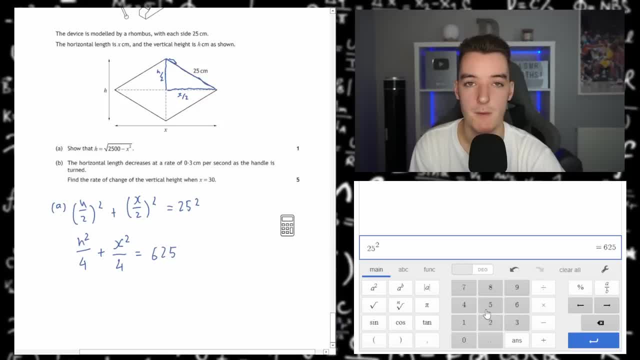 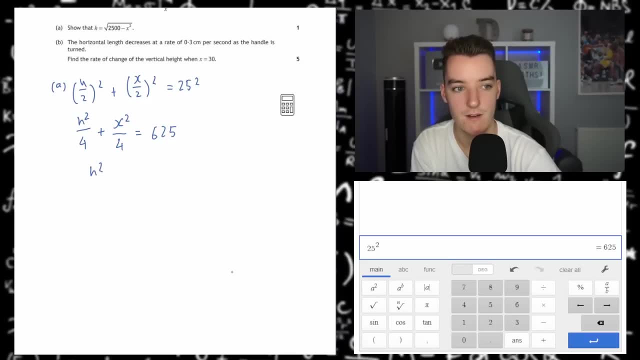 it by 4.. Because we're going to multiply everything through by 4 to get rid of the fractions, which gives h squared plus x squared equals 2500.. So h squared is equal to 2500 minus x squared. So h is equal to the square root of 2500 minus x squared. 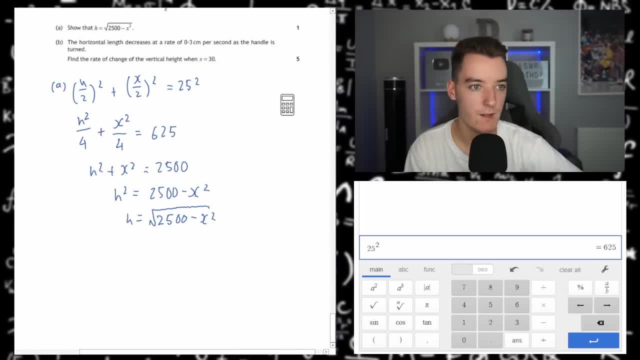 ome, Huh, Oh no, that's good Birds, Wherever you are. Oh, I guess I'll say: I'm good And there we go. that's what we're asked to show. What does part B ask us to show? 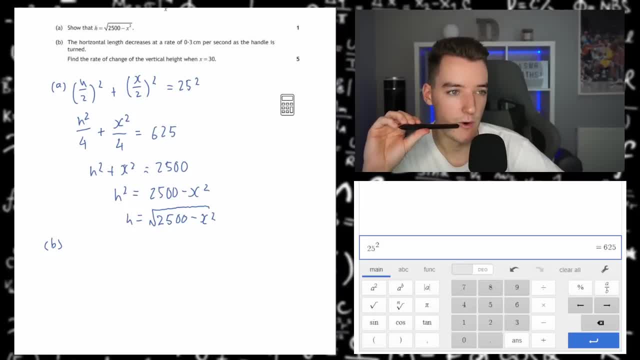 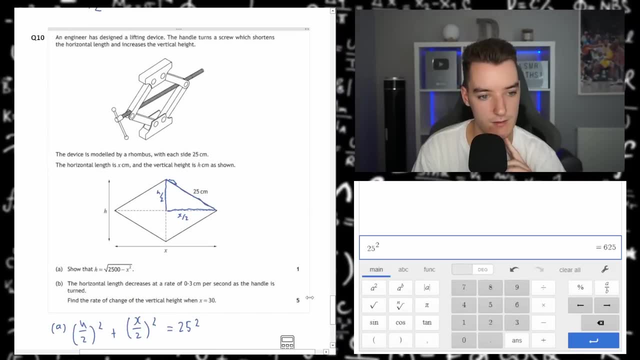 Worth five marks, by the way. The horizontal length- let's get the entire diagram back up. So the horizontal length decreases at a rate of 0.3 centimeters per second as the handle is turned. So as the handle turns, the horizontal bit decreases. 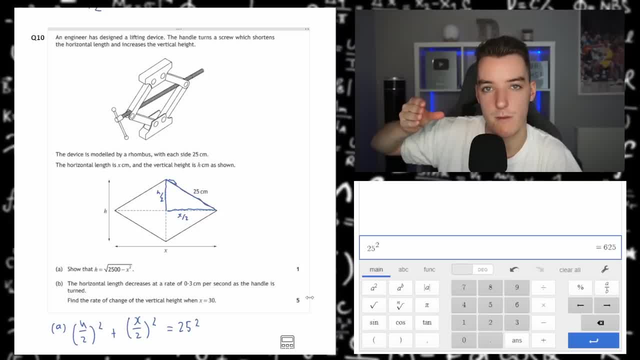 Oh, horizontal decreases by 0.3 per second, whereas the height will change. in relation to that, We want to find the rate of change of the vertical height when X is 30.. Okay, that looks like a lot, That's a lot of information, but we can do this. 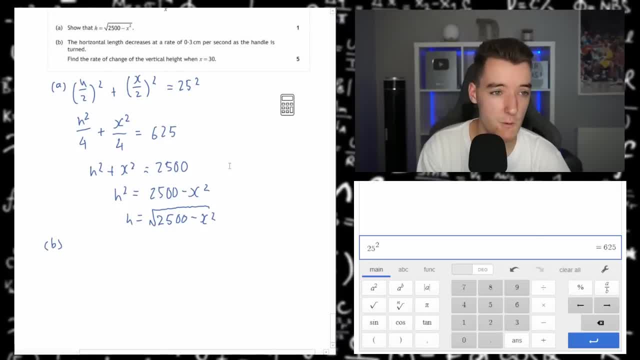 We can do this. So we know that the rate of change of the horizontal, which is just dx by dt, is negative 0.3.. So we want to work out the rate of change of the vertical, We want to work out dh by: 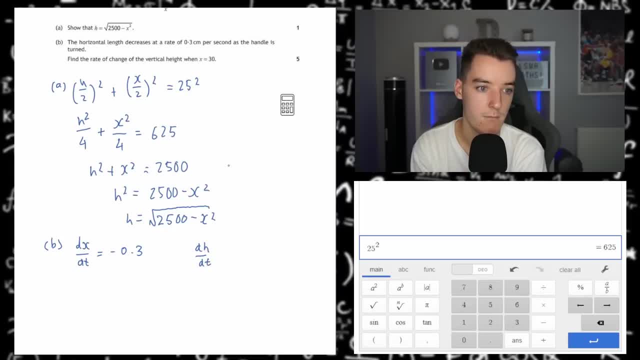 dh by dt, But we have h in terms of x, So dh by dt. I can see how this is going to work. It's simply going to be dh by dx multiplied by dx by dt. So if we can work out dh by dx, 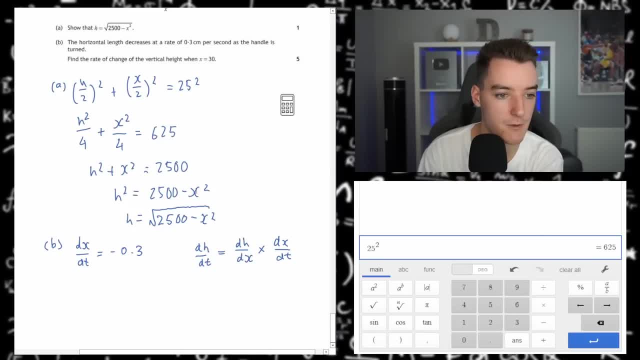 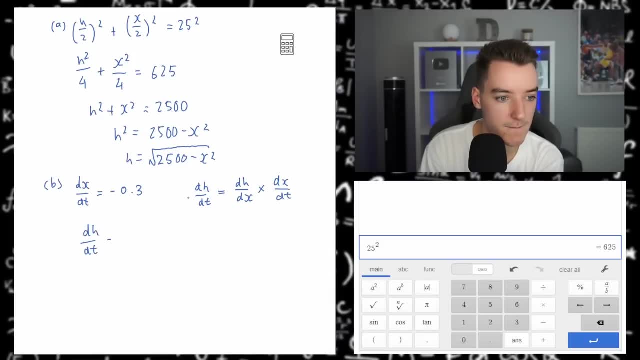 we can work out dh by dt Pretty simple. Well, let's do it. dh by dt um. well, we know h um. i'm actually going to rewrite this as 2500 minus x squared to the half, because that's what the square root is. so, differentiating this, we get a half. 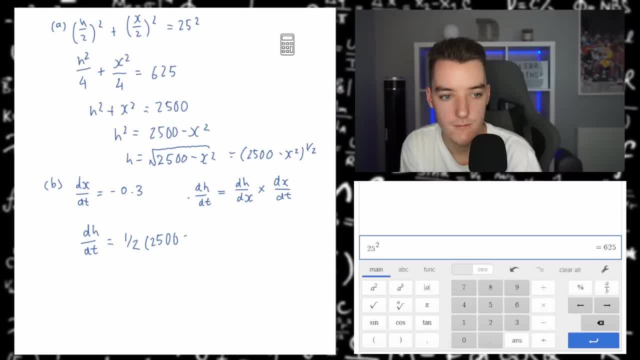 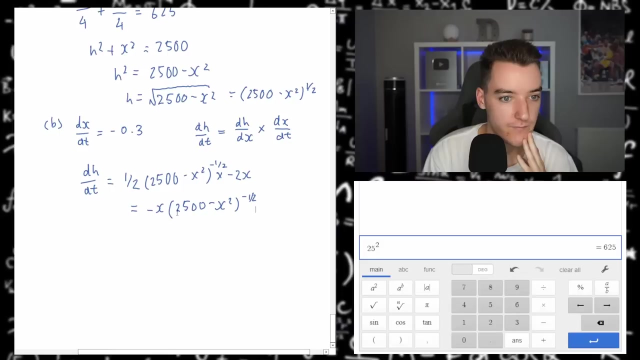 2500 minus x squared, multiplied by negative 2x, and then decrease the power, so this gives us minus x, 2500 minus x, squared to the power of negative a half. um, sorry, this is. this is actually probably a really tricky question. so now to work out. oh sorry, this is dh by dx. 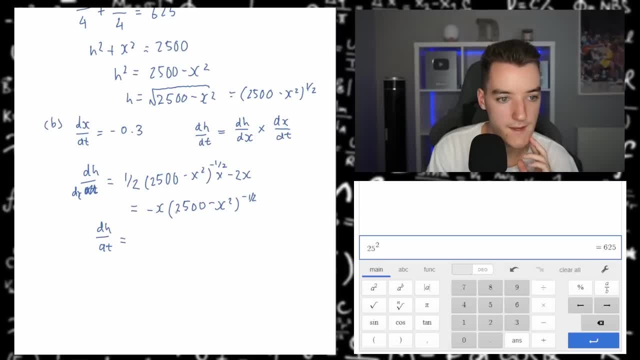 so dh by dt is equal to this thing here multiplied by minus 0.3. so that's going to give us 0.3x two-thirds and 500 minus x squared to the negative a half. and then at what was it the rate of change when? 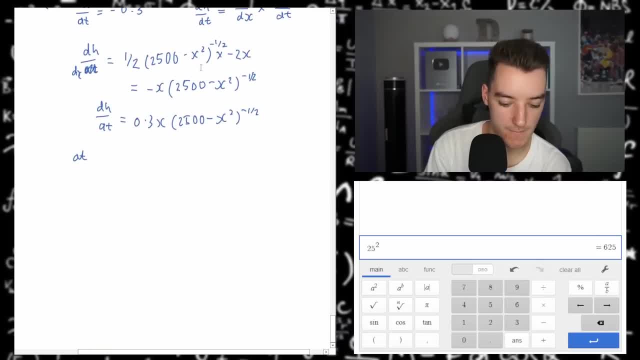 the vertical when of the vertical height. when x is 30, so at x equals 30, the rate of change of the vertical height- let's just use a calculator- is going to be 0.3 per minor times 30 times. let's do this bit in brackets. do that as in: 500 subtract 30 squared to the power of negative a half is zero a point. let's convert it to a fraction instead: 9 over negative a half. lets convert z to a fraction instead 9 over negative a half is zero point. let's convert z to a fraction instead 9 over negative a half is zero point. let's convert z to a fraction instead 9 over line, halving it over to community instead massive. 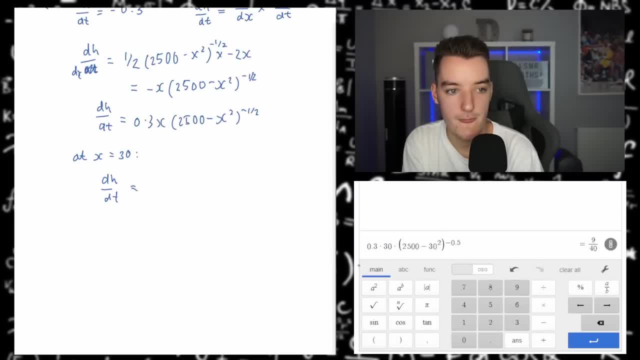 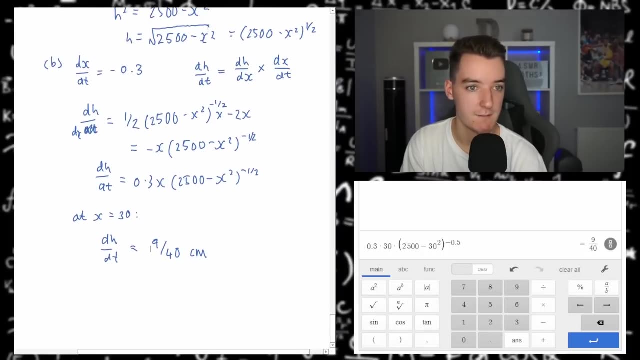 instead 9 over 40 centimetres. That was actually a really tricky question. I had to piece together a lot of things there. I think this bit here kind of was lucky that that popped into my mind, Very lucky we're allowed to use a calculator too. and yeah, definitely the hardest question. 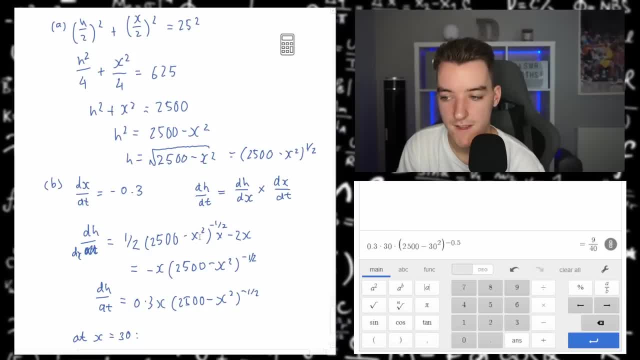 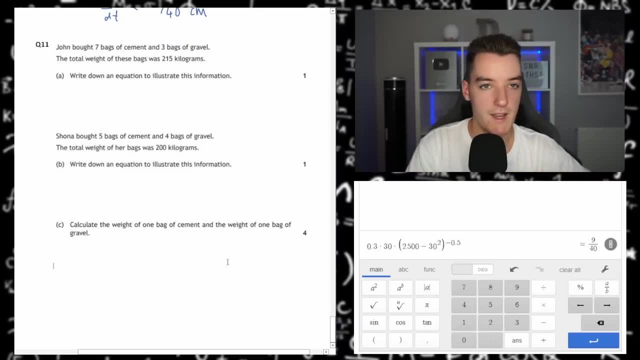 we've done as of yet, But we'll move on to the next one and see how things progress for the last couple questions of the video. Okay, so question number 11: here Looks like a little bit of simultaneous equations. John bought 7 bags of cement and 3 bags of gravel. The 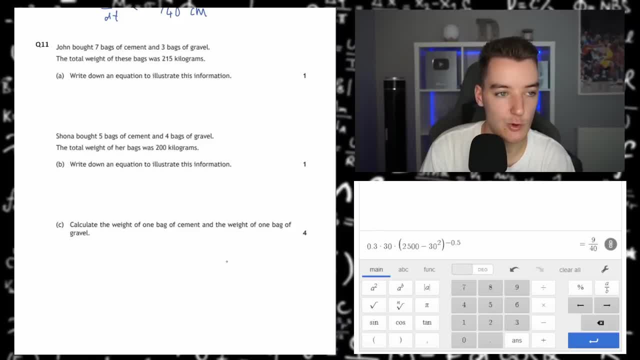 total weight of these bags was 215 kilograms. Write down the equation to illustrate. So 7 bags of cement plus 3 bags of gravel is equal to 215 kilograms. Sean bought 5 bags of cement and 4 bags of gravel and the total weight was 200.. Nice, Very easy these first. 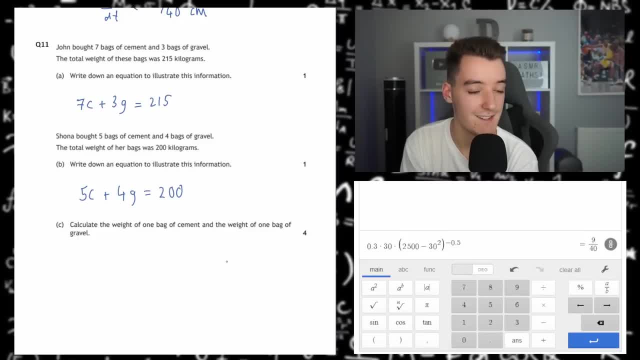 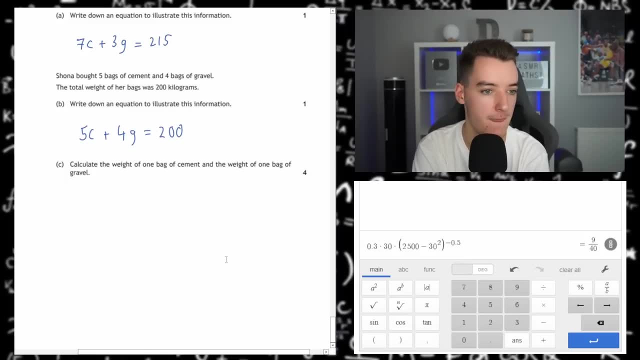 two marks, And that's the equation to illustrate that- And part C. I know I've rushed those first two parts, but part C is the bit where we need to do some thinking. So calculate the weight of 1 bag of cement and the weight of 1 bag. 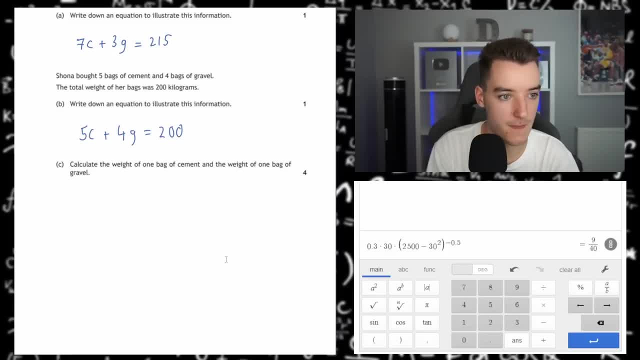 of gravel. Okay, so let's take these equations, Multiply the first one by 4 and the bottom one by 3.. So let's call these 1 and 2. Like so. And when we do this for the top equation, we're going to simply get: 28C plus 12G is equal. 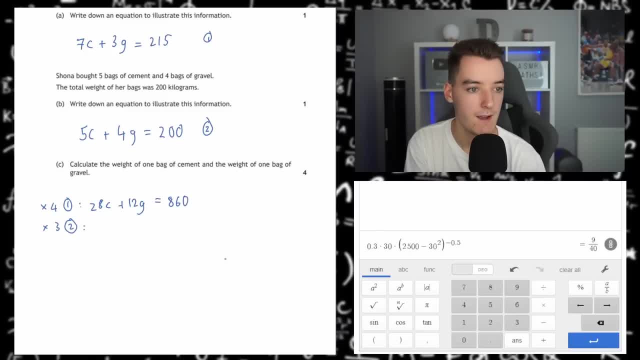 to 860. And the bottom one's going to be 15C plus 12G is equal to 600.. Subtract the 2 and the 3 and get 13C is equal to 260 or C is simply equal to 20.. So when C is 20, substituting: 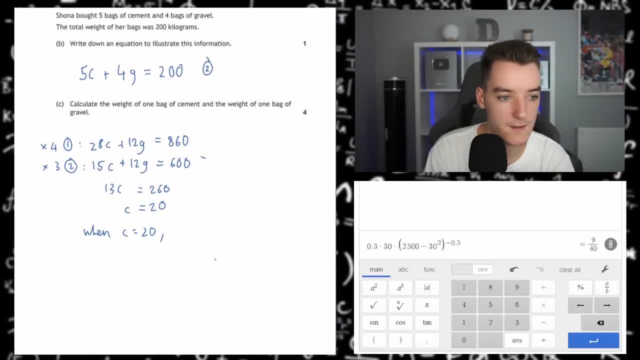 in, OR I'll put sub into 2.. So if C equals 5 and 6, we need to subtract yet again 18C plus 2.. emmm, Two times 20 is about 1000.. I don't have this, Who knows. That's kind of still missing. 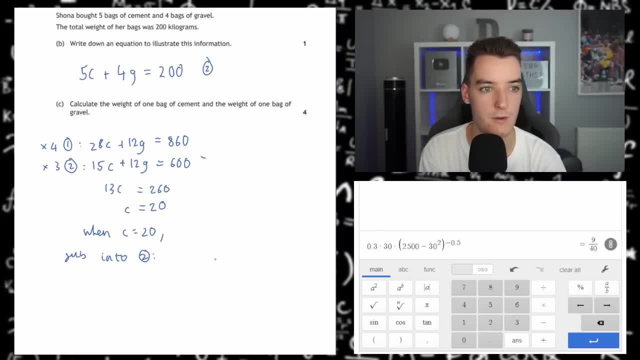 anywhere at least. Uh well, that's easier than on the law teacher, I can put That right. 81, that's speculation. Simplify c is 20, we're going to get 5 times 20, which is 100, plus 4g is equal to 200, or 4g is. 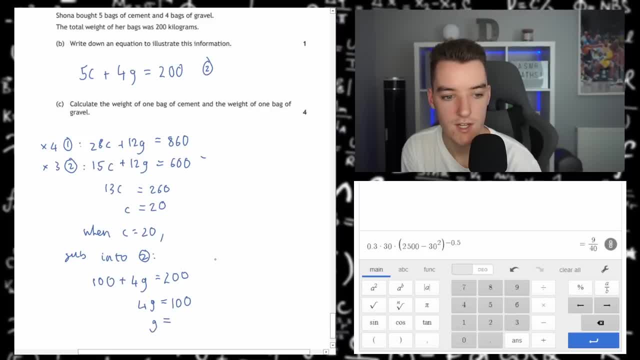 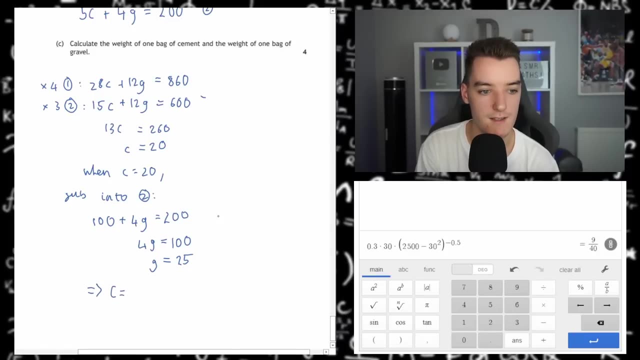 equal to 100, or g is simply equal to 25.. And there we go, We have worked out the weight, And let's just do a little bit at the bottom, where we say, therefore, c is equal to 20 kilograms, g is equal to 25 kilograms. Very nice question. I've said they're all very 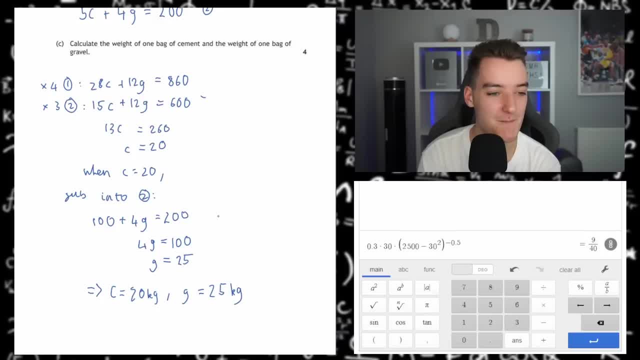 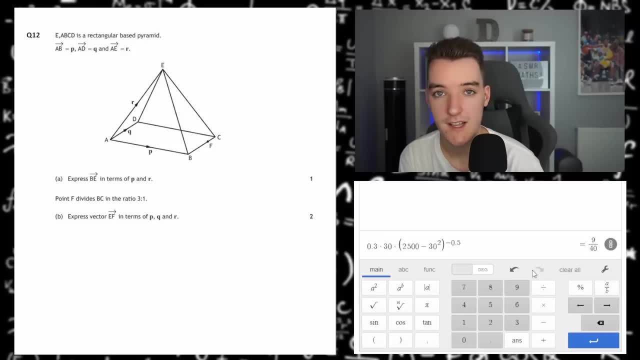 nice questions, but that's because I love them. Speaking of which, let's go on to our very last question of the night. Well, have you voted? Have you fallen asleep yet? Maybe you have, or maybe you've made it to this point, which? 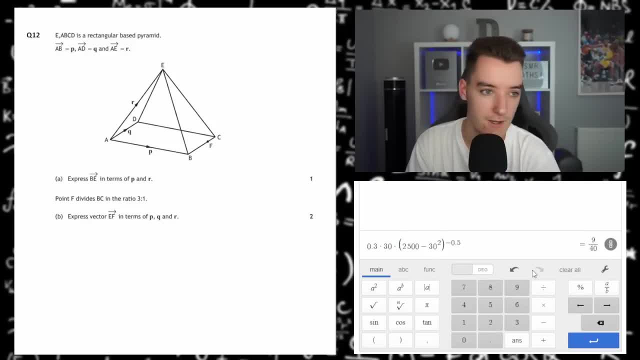 is going to be the last question of the video. looks to be a bit of geometry 3D geometry. E-A-B-C-D is a rectangular based pyramid with the vector A-B expressed by B, A-D expressed by Q And A-B-C-D is a rectangular based pyramid with the vector A-B expressed by Q and A-D expressed by M. 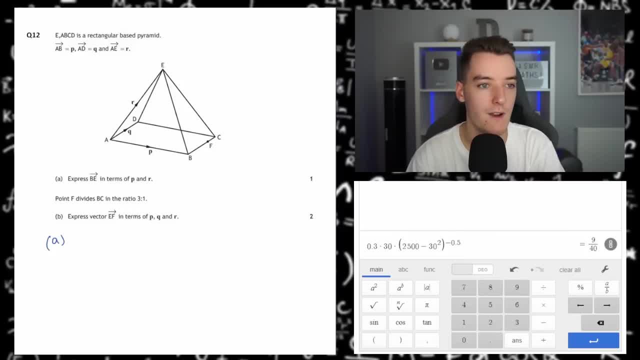 A, E expressed by R, We are asked to express B- E in terms of B and R, so B to E, which is up there. Okay, so how can we work that out? Well, we can go back along A, B, which. 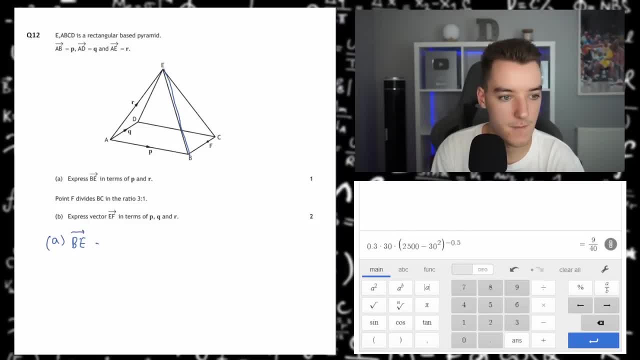 is minus B, and then we can go up A E which is plus R, so minus B plus R, or we could just do R minus B, which works the same. But there we go. that's part A, part B Point. 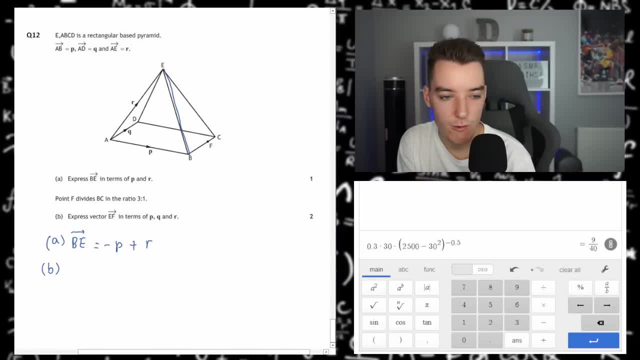 F divides B- C In the ratio three to one. express vector E to F in terms of P, Q and R. Okay, so we want to try and go from like here to here Now, because it divides B- C in the ratio three. 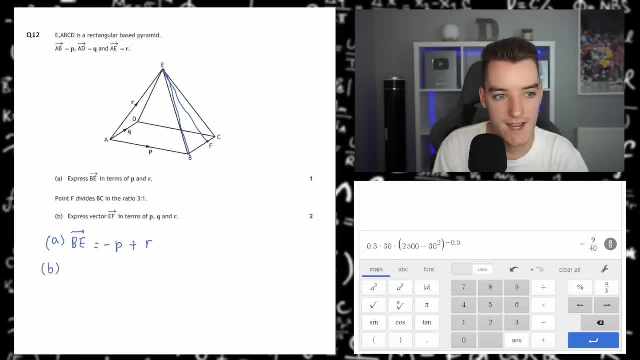 to one. B, C is the same as A, D because they're parallel, I think. So it's going to be three quarters Q at one point, So we could go back along A, B, Q. let's write this as EF. what we know actually to get from B to E is minus BR. 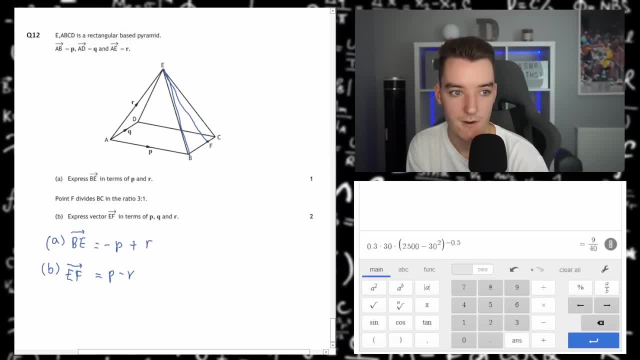 so the opposite is just going to be B minus R. I'm pretty sure, yeah, B minus R, and then we're gonna plus three quarters Q, and that should be how to get there. yep, looks good to me and that is gonna be the final question. hopefully I got. 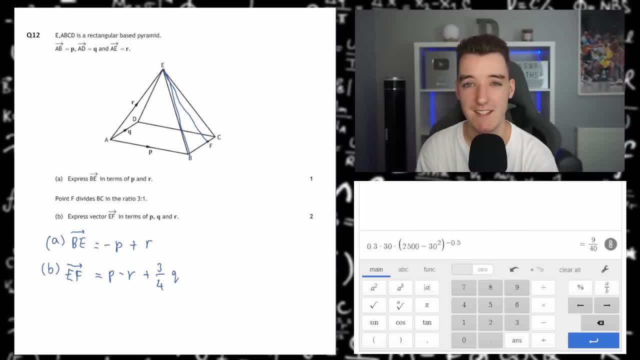 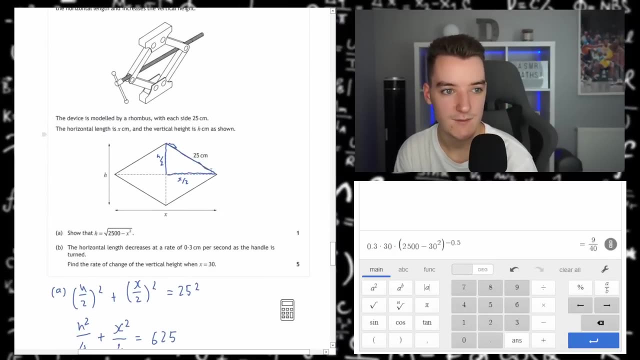 them all right. if you guys have noticed any little mistakes I made, I do apologize, but feel free to let me know in the comments. and, yeah, let me know what your favorite question was as well. from all these questions that we did take, I think my favorite, I like this one. 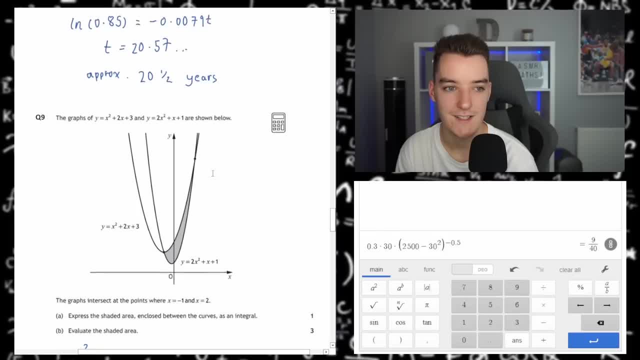 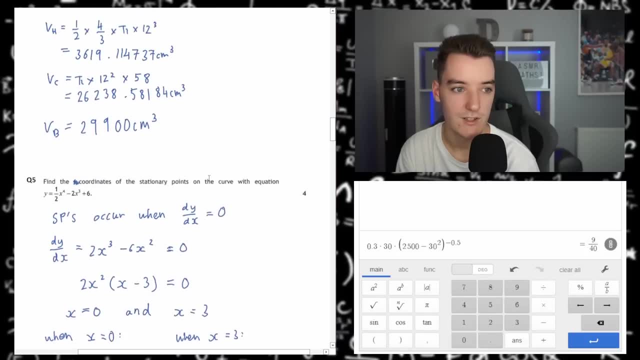 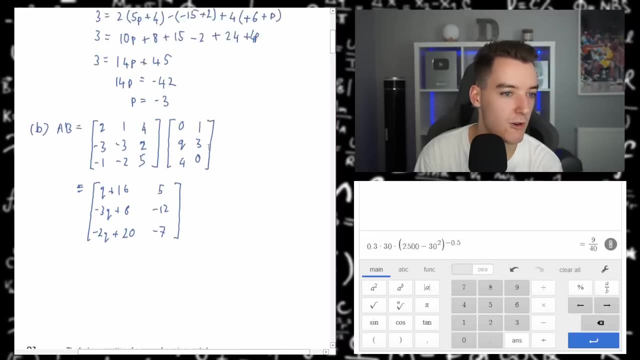 I think this was a fun question. question ten: what else did I like? I like question eight. question six was a good. question five: we added our fun little twist and, yeah, they were all good. they were all good. question one was fun as well, guys, that is where 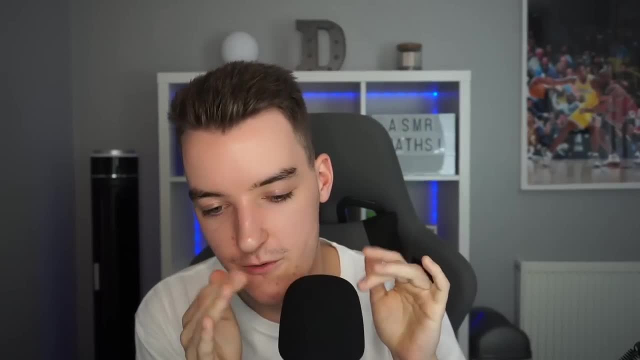 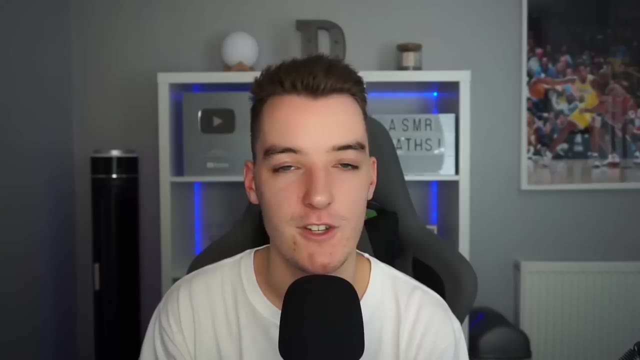 we are going to bring tonight's video to an end. I really hope that you all did enjoy and if you did be sure to drop this video, a big thumbs up. let me know if you made it to the end without falling asleep. I really hope you did. 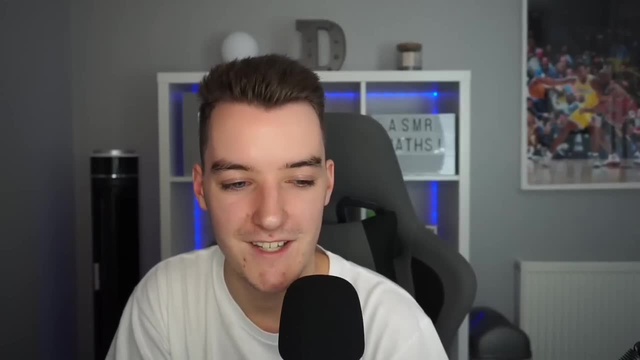 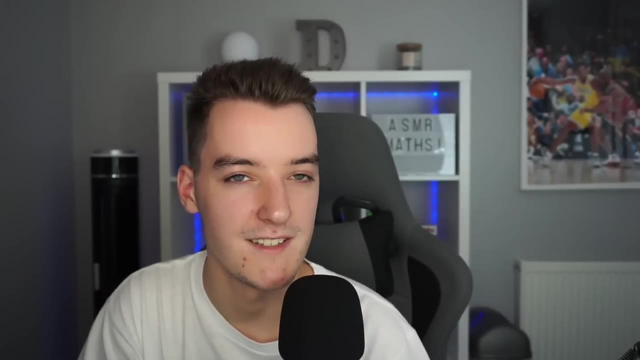 because that was the aim of this video- was for me to try and make you fall asleep whilst doing some relaxing math puzzles and problems, so I hope you did and I'll see you in the next video. bye, bye. so I hope you found that the problems nice and satisfying and enjoyed this super extra. 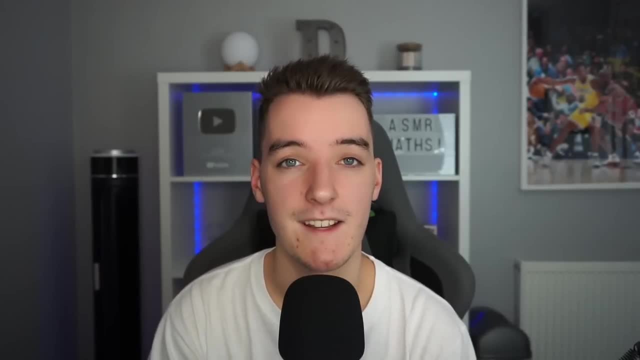 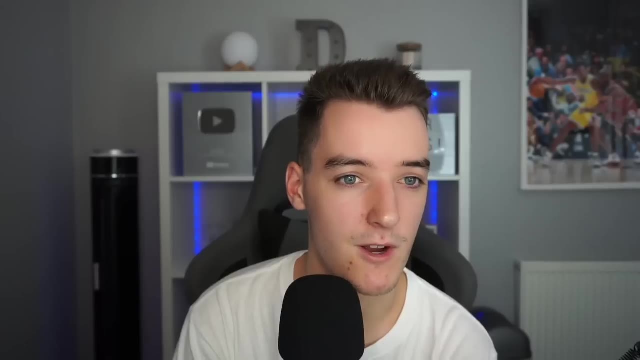 long asmr maths video. I love making these. they take a long time to make, so I put a lot of work into these and I want to say a huge thanks again to my girlfriend for setting up the questions. let me know if you want to see more asmr maths or as maths are, and yeah, 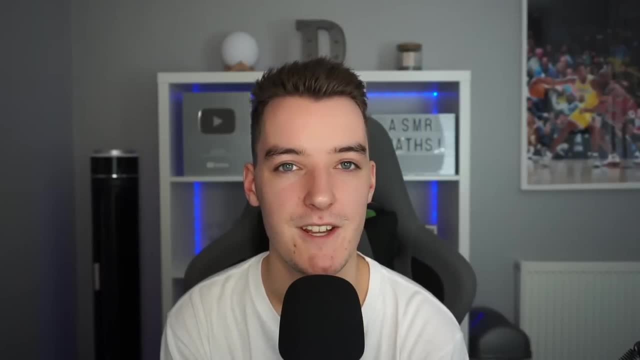 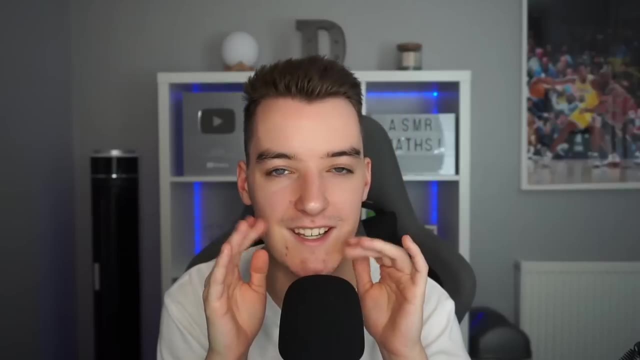 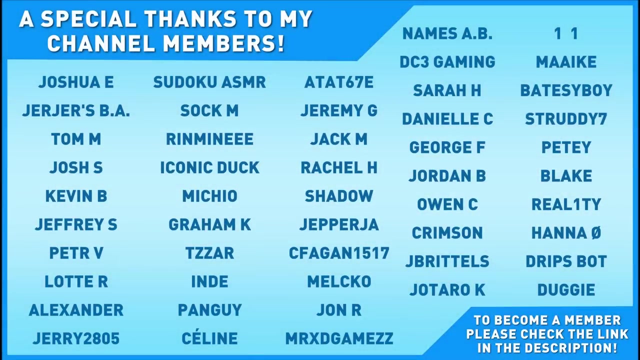 appreciate all the support and I'll catch you all in the next video. goodnight everybody, goodnight everybody. a quick thanks to the members of the dido asmr community. thank you all so much for becoming a member.